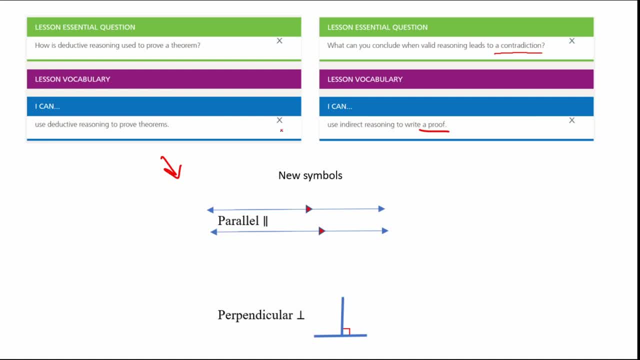 writing assignment. But to do that, I'm going to introduce some new symbols, And these are symbols that we're going to need for today's lesson and for tonight's homework. Your first new symbol is parallel in the textbook. It'll look like that When I write it: handwritten. they're usually 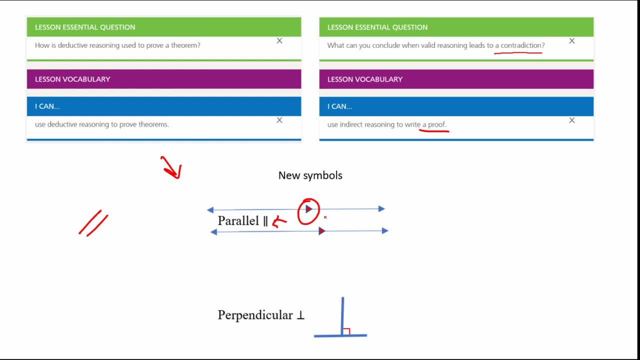 slanted lines And when I write it they're usually slanted lines. And when I write it they're usually slanted lines And symbolically they look like that on a line, But more likely they're going to look like this. They're just arrows at that point. So this means these are parallel. These are no longer. 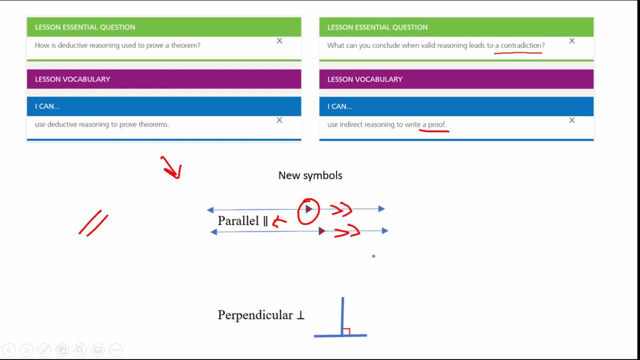 parallel. Just like the tick marks, the number matters, And now they're parallel again. So let me show you what that would look like. So let's define this as line one And this one is line two. Because of these marks right here and they're the same number, I can say line one is parallel. 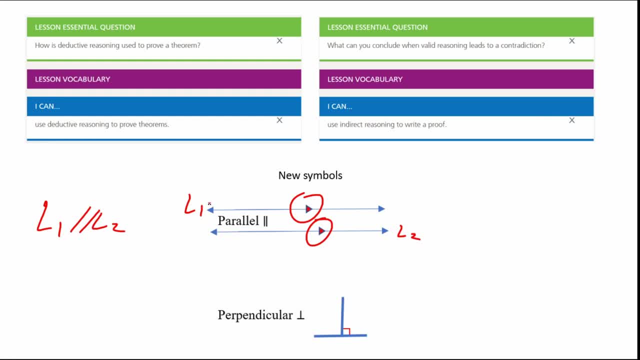 to line two, And parallel just means they will continue. Since they're lines, we know they continue forever in both directions. But parallel means on a flat surface they will never intersect In quarter three. if you're doing really well in the class and you want a harder challenge for your writing, 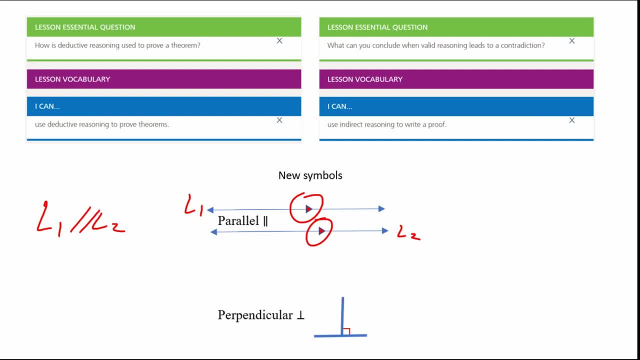 assignment we will look at curved surfaces and why our definition of parallel doesn't actually fit all cases. That's a much more advanced topic. I have had a few students tackle it and they've done fairly well. You get a lot more leeway in that writing assignment. That is purely an effort assignment. I'll get more into that as we get. 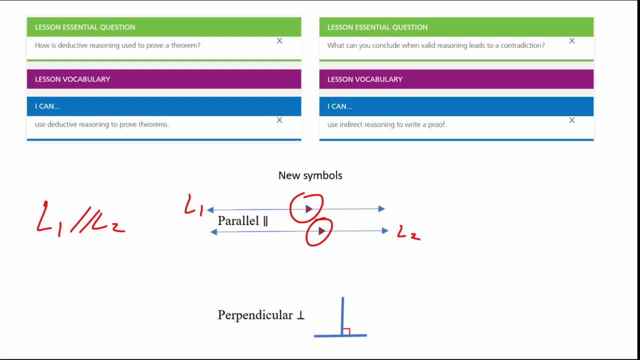 closer to the third quarter writing assignment. But if this has piqued your interest, keep this in the back of your mind and come talk to me about parallel lines on non-Euclidean surfaces. Alright, let's talk about perpendicular lines. So perpendicular lines meet at 90 degrees And there's some nice. 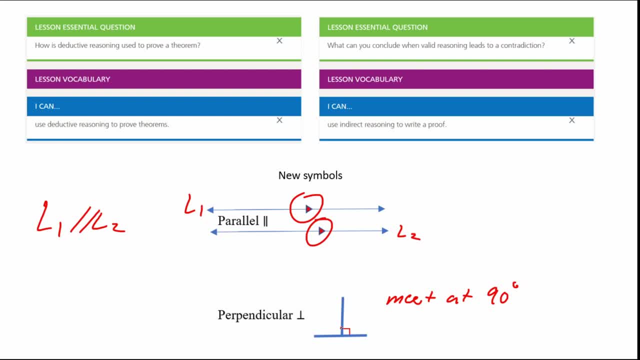 things about that, And that is, we know that the measure of this line here is 180. So if this is 90, this is 90. We also know, if we were to continue this, this would be 90 and 90. So this shows us, if we all go all the way around, 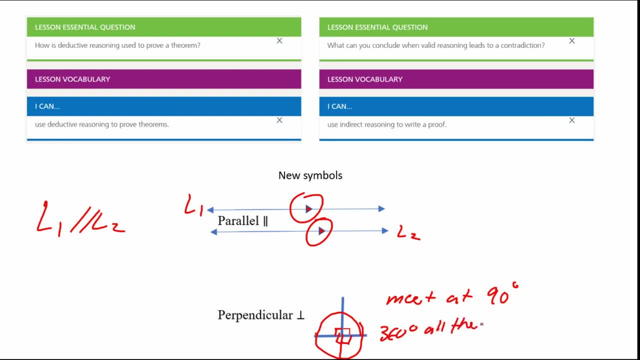 we get 360 degrees And, if you didn't know already, a circle is 360 degrees. So there is a little bit of a visual proof of how this works on a coordinate plane and why a circle is 360 degrees is 360 degrees. but most importantly is that you know this symbol right here. so 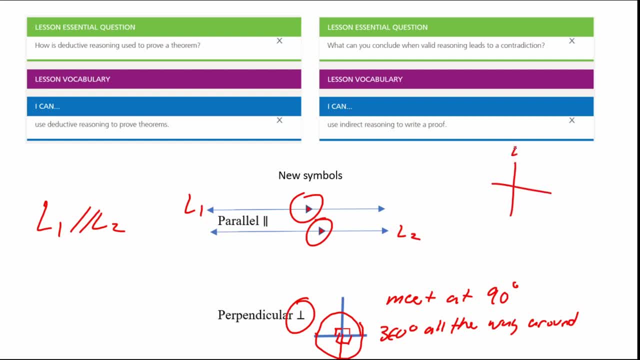 now let's draw two more lines. let's call this line three and line four. what you'll see me write is: line three is perpendicular to line four. so there's our new symbols for today. let's move on to the actual lesson. next slide, we're gonna look at a two column proof. you will do a minimum of three of these on. 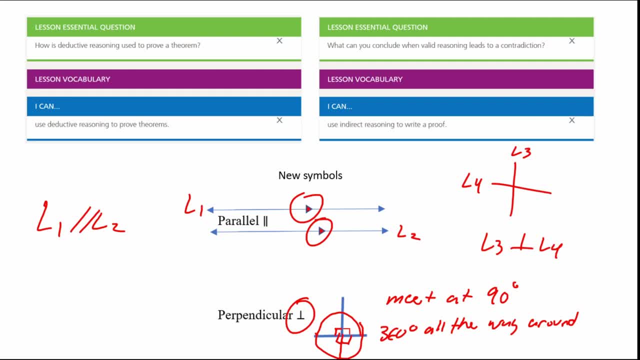 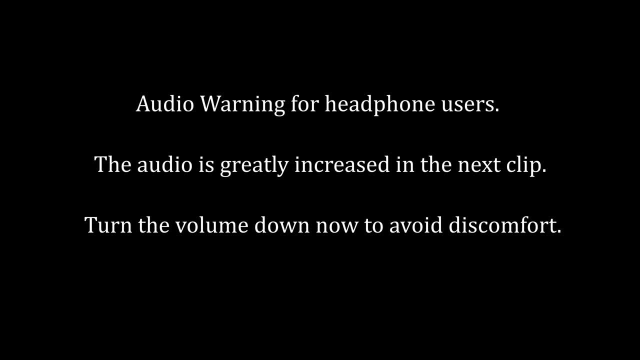 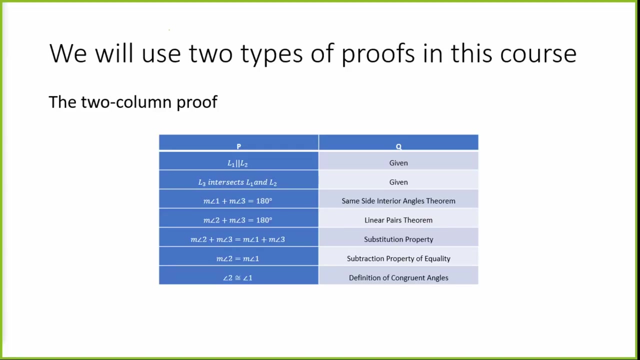 your writing assignment next quarter. let's look at our two column proof. this is the first style we'll learn in this course. it's called a two column proof because it is two columns: it's a hypothesis column on the left and a conclusion column on the right. remember, P is always your hypothesis and Q is always your. 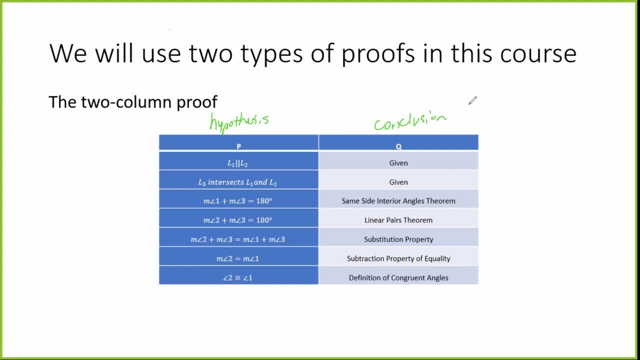 conclusion. now let's look at, let's just read it and you'll see that what I meant by writing mathematically and being a big part of this course, it's kind of looking us right in the face. here we have here is line one is parallel to: 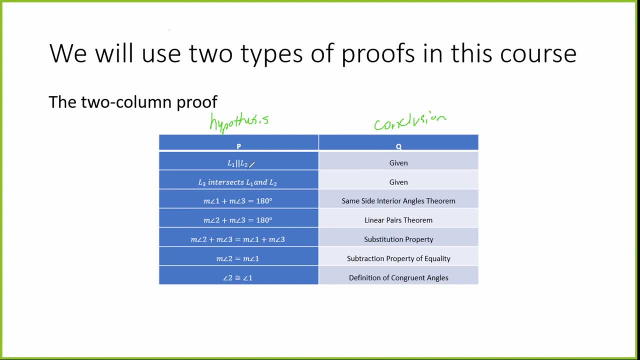 line two and that's our given right. that means it's from our hypothesis. line three intersects line one and line two. that's also given. so let me draw that and show you what that would kind of look like on our problem. we're gonna reverse engineer this, so here's a line and here's a line, so we'll call these. 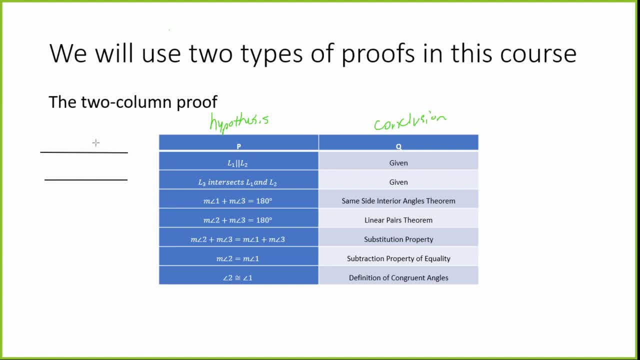 line one and line two, and we know they need to be parallel. so I'm gonna go ahead and add a parallel marker to each one so that we can see that that's what's given. and if we were given this and we were to say, put this information into a, 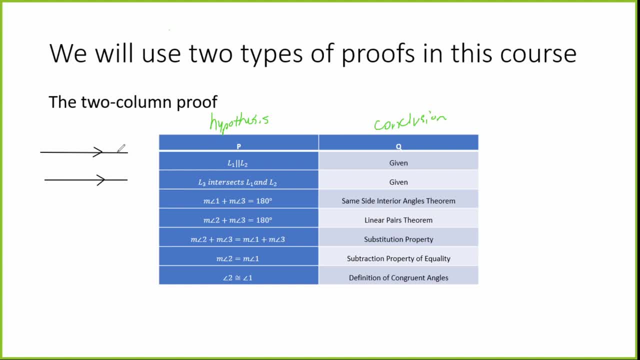 two column proof. once I have labeled the lines, we can go ahead and do that. so now we have line one labeled, we have line two labeled and we have shown that they are parallel. so here is everything here. so what this would look like written in a conditional is: if line one is parallel to line two, of course we'll have. 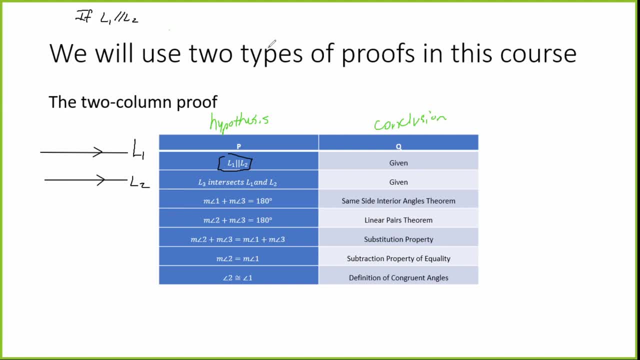 that written out in full sentences, but for brevity let's leave it like this: so, because it's in our hypothesis, it goes after the if but before the then. and then we have line three intersects line one and two also given. so then we're going to say: and line three intersects line one and line two, so we need a third. 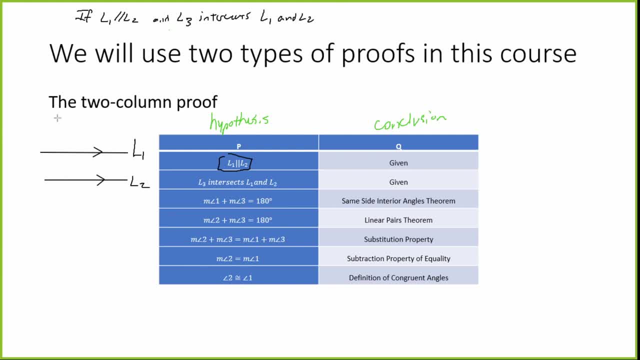 line here. I'm going to go ahead and draw that third line in and that line intersect. notice, it doesn't tell you at which angle it intersects, so we don't have to worry about that and we can't add that information yet. right, because it's not. 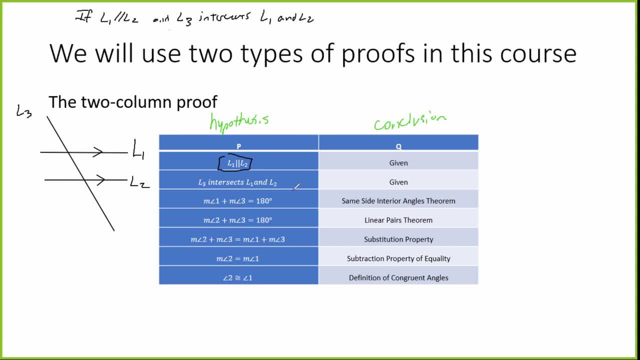 in the given. so I'm gonna call this line three, and so far we've now reverse engineered our hypothesis. and then, if we want to look at it again, if I just started with this diagram, I would just say what was given in the diagram. line 1 is parallel to line two. 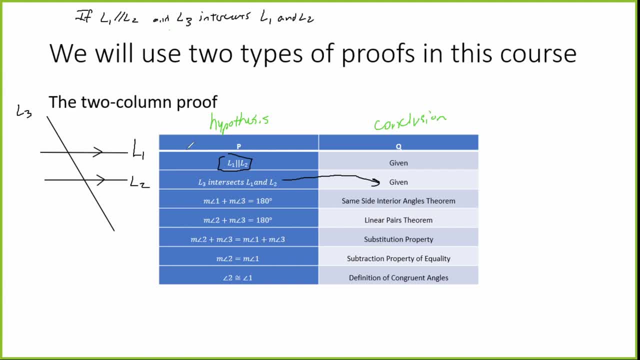 line three intersects it both lines and it doesn't say anything about the angle, so i haven't added any additional assumptions here. i'm going to change the color of my ink so we can talk about what we want to do. what this one is going to do now is: i want to look at my conclusion. 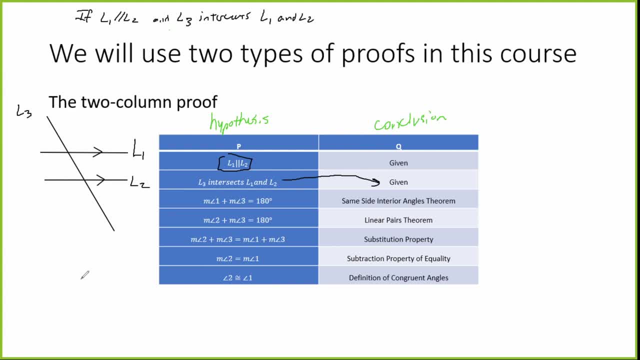 and my conclusion is always my last one whenever i have my then part. that's what we're working towards, and if we can start with our hypothesis and use known theorems, sometimes postulates and conjectures, i wouldn't do that for anything too serious, but if you just 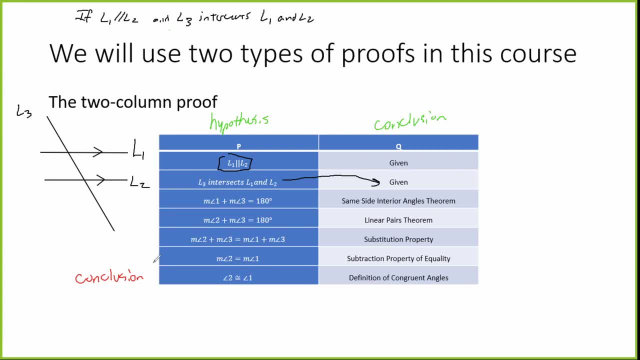 want to try and get from point a to point b, then we have to go back and look at our postulates and conjectures and try and do a proof of them to avoid them at all costs. go with the same, with um knowns in math classes, theorems that we cover in this class, because we know theorems are. 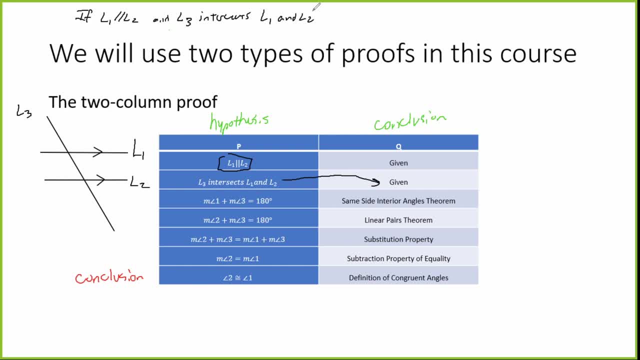 always true, but our conclusion is then: angle two is congruent to angle one, so now we need to label these, and the nice thing about this is: this is what we're concluding. right, this is what we're saying. so, on this diagram, i have a little bit of freedom here to label. 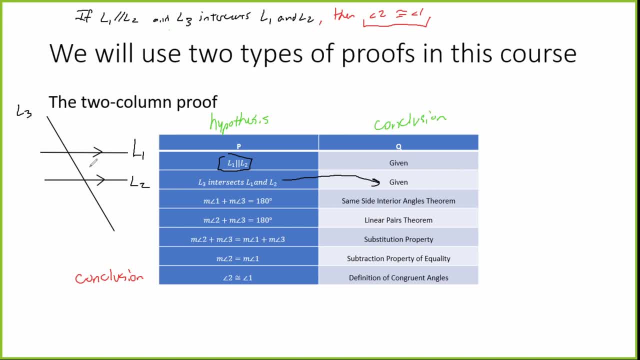 this, however i want. however, if i mislabel it, then we're going to show that we have a contradiction or that it's not true, so we need to be careful in how to label it. what we want to show is that one is congruent to two, so what i'm going to do now is take a minute and look at this. 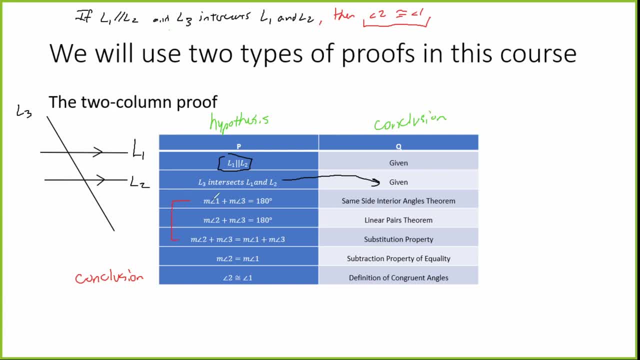 and see if i can reconstruct this drawing to match this. this is not something you'll have to do, so i will give you the positions under root 3-nov. so i will give you the positions under root 3-nov. so i will give you the positions under root 3-nov. so i will give you the position. which one is correct? shut down and open, execute uret al geven. so we'll take the options and give you the position e. then you're going to doformation. so these are our examples. which one is correct? lets do everything you want to do. i will give you. 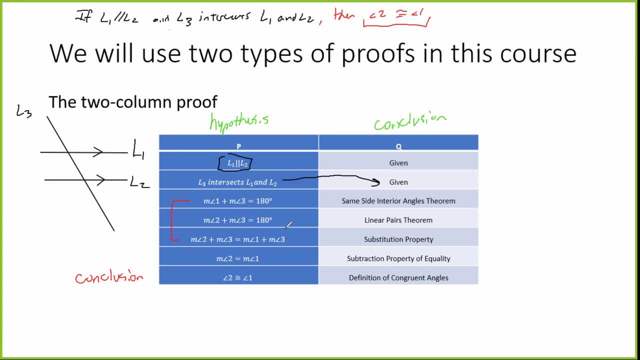 the positioning of the angles and just ask you to prove it during this chapter. in chapter two you're going to have to do a little bit more of the lifting, but i have some knowledge right now that you don't with this theorem here. we know this one and you guys should know everything. 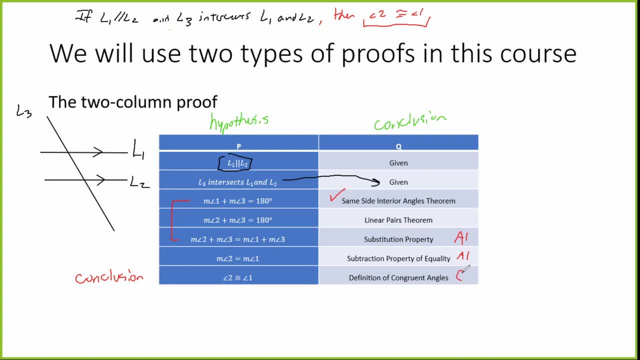 else from either algebra one or in my class so far. so the same side interior angles me. theorem tells us that if we have two lines that are parallel, then we have two angles on the inside of those or on the interior who are on the same side of the transversal line. three is called the 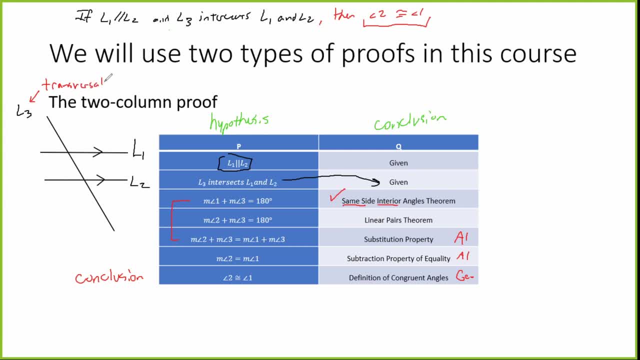 trans versal and all the transversal means is: it passes through a line, two lines, three lines, a number of lines. it transverses them. so if i break this down one more time, same side of the transversal and on the interior of the parallel. we have a symbol for that, so i'm not going to spell it out. 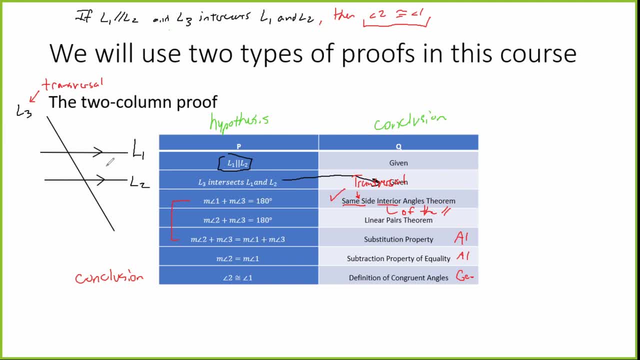 anymore. so same side of the transversal and on the interior. so here's my parallels and i can either use this side or this side of the transversal. so again, i have a lot of freedom here. but i'm going to go ahead and pick this and this for one and three, and then i'm going to look at this right. 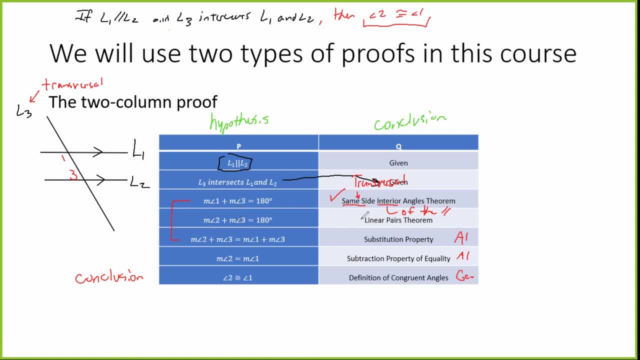 here and it tells me that angle two plus angle three by the linear pairs theorem. well then, now there's only one place that can go. well, actually, there's two. right, it can go here. or it can go here because it can be a linear pair this way, or it could be a linear pair this way. i am more inclined to naturally choose. 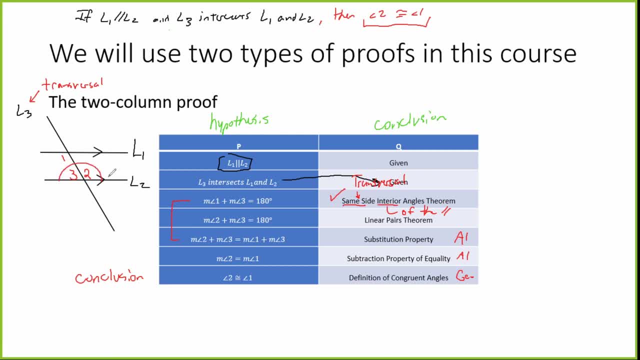 this position only because the line is horizontal and it's easier for me to see it in that fashion. so now i'm going to look at my next step and we're just trying to prove that angle 2 and angle 1 are congruent, and to do that we need to see if all of these steps hold. 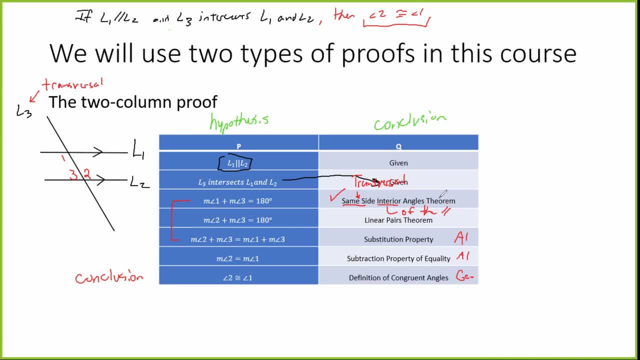 true. well, another nice thing about the same side interior angle serum is that the two angles equal 180, and we'll actually prove that in topic two, but for now i just want to show you how this proof works. so the measure of angle 1 plus the measure of angle 3 does equal 180 by the same side. 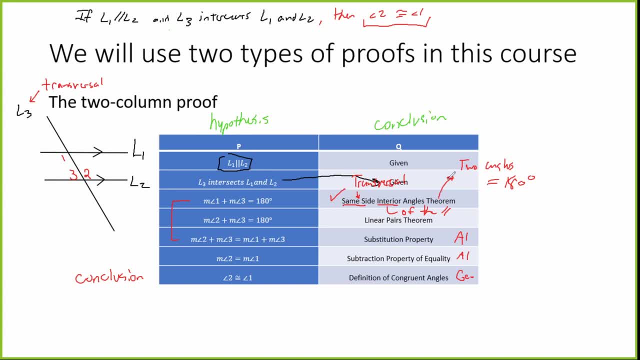 interior angle serum. so when you're writing your proof you can kind of see now that in algebra- and this is what i kind of told you- it was going to be so different about this class- in algebra we're going to give you that angle 1 is maybe 120 degrees and angle 3 is 60.. and we're going to say: 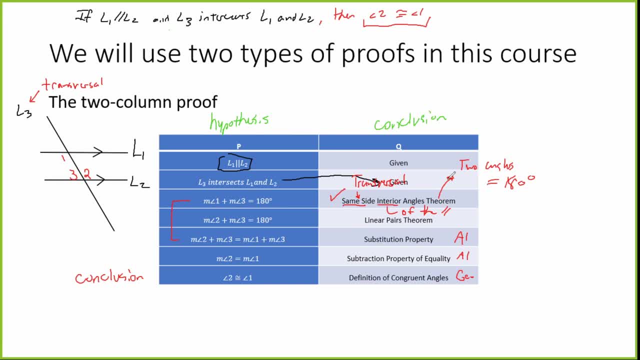 can you solve it? or we're going to say angle 1 is 120 and angle 1 plus angle 3 equals 180.. here we're doing it for any number, and this is where we start talking about generalizing what we're doing. all of this is very generalized. we can plug in any number for angle 1 here. 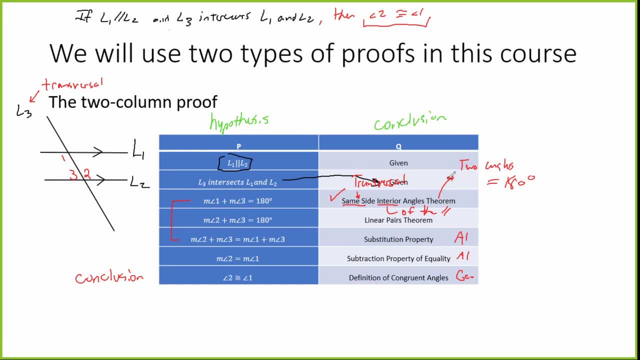 and solve for angle 3 and it holds for any value of angle 1 or angle 3.. this is why it's called a proof. it works for any value if we can follow these steps and show all of them to be true for this case. if we adjust the transversals angle, then it will be true for all cases. 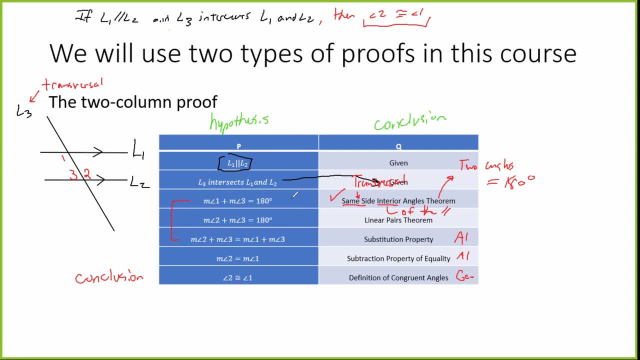 so this one checks out by the same side, interior angle serum, measure of angle 2 plus the measure of angle 3. this one you're ready to verify. we know about the linear pair serum and we can see it right here and we've already kind of drawn our protractor of 180 degrees so we can say this one's. 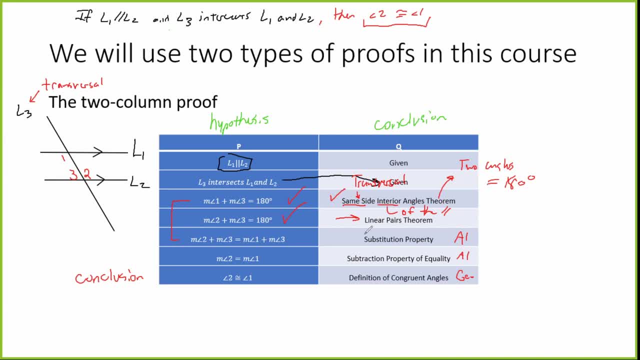 true. now this is a little bit of an interesting one. this is a substitution property, right? if two things have the same value, i can substitute them in for each other. well, if the measure of angle 1 plus the measure of angle 3 is equal to 180 and the measure of angle 2 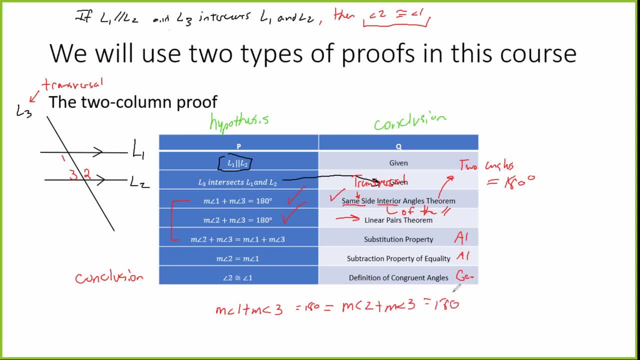 plus the measure of angle 3 is equal to 180 and remember, this works for any measure of these two. they're locked together as this line rotates right if it come. if it had come in at any other angle by the linear pair serum, it doesn't matter what that angle is. 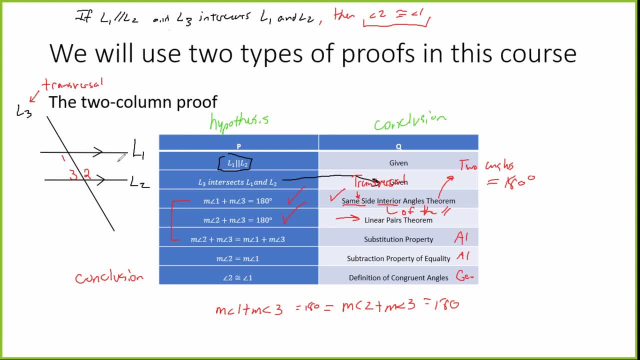 they'll still be 180 degrees when you add them together. so one thing we can do here is, if they're both equal to 180, we can remove that value, because we have our variables here and we end up with measure of angle 1 plus the angle 3 plus the measure of angle 2 plus the measure of. 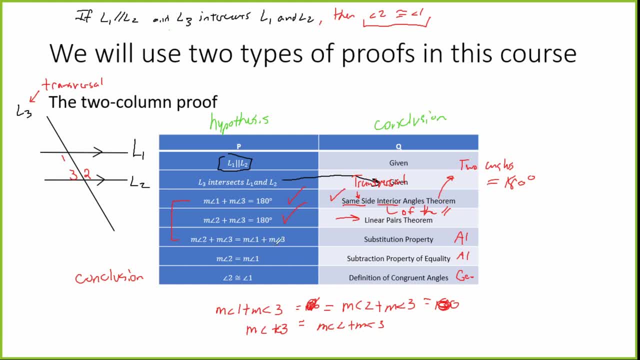 angle 3 are equal. well, we can then subtract angle 3 from both sides because they're the same value. so we can balance the equation through the substitution property. we can then subtract the measure of angle 3 from both sides, and since the measure of angle 3 will always be equal to 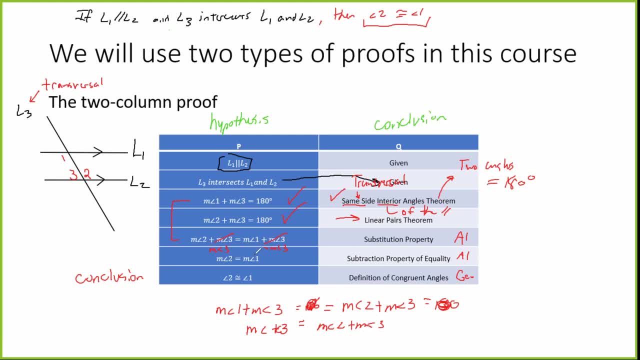 itself. it leaves us with: the measure of angle 2 is equal to the measure of angle 1 and that to get to that step we had to do the subtraction property of equality, and what we were shooting for here is that angle 2 is congruent to angle 1, and that is the definition of congruent angles. so i have a few more of these two terms. 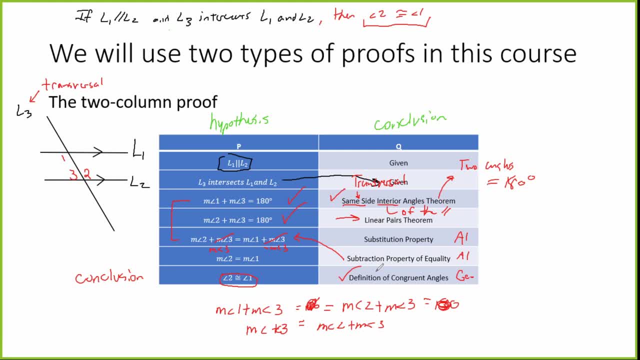 show you as we get going. but the whole idea here is to get the spirit of the two column proof down. it is a: you always start with your hypothesis as you're given and then you move into any steps necessary to get closer and closer to your conclusion. 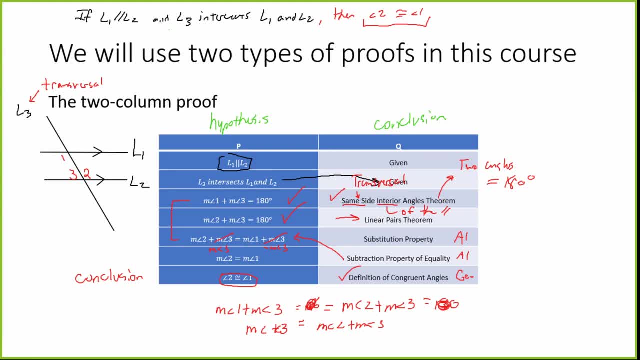 until it is all said and done. so a recap: this was given by a diagram. this was given by diagram. it could also be given by a sentence, like i had above, and then all of these theorems were used to prove this step. now, one thing that i do, and i'm not going to require you to do, because 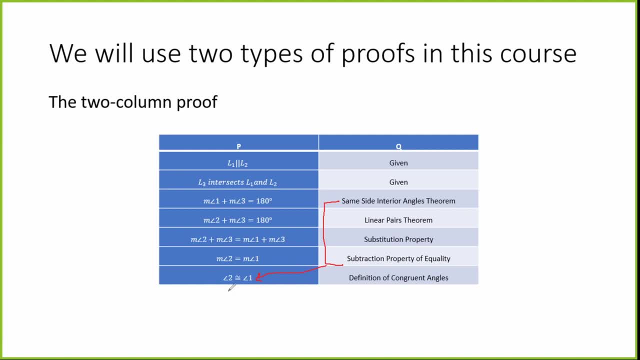 not all proofs do this and this was just something from the university that i came from. they would make me rewrite this and then here, because i started with a given, i would write conclusion. now i asked one of my professors- why, dr garman? and he told me that way. i know you thought you were done, or you're. 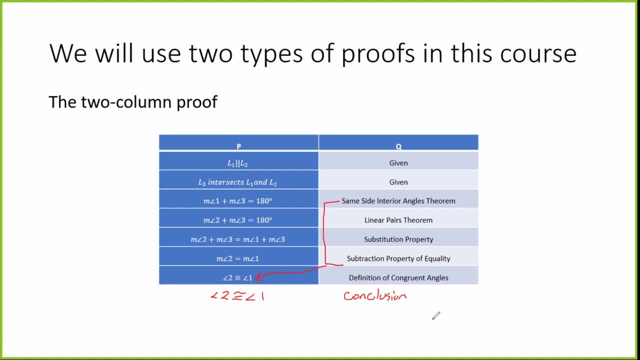 telling me you're done. so if you missed anything or if there was another step, i could provide you more accurate feedback by saying: yeah, you're almost there, but you're not quite there. it's going to look great on your paper if you go ahead and do that for me. i know it's an extra step. i'm 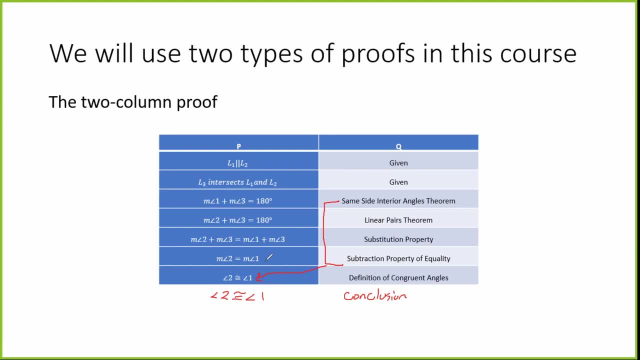 not going to hold it against you if you don't, but it does to me and in the very few books that i've seen it offer a more accurate answer to that question. i'm not going to hold it against you if you don't, but it does to me and in the very few books that i've seen it offer a more. 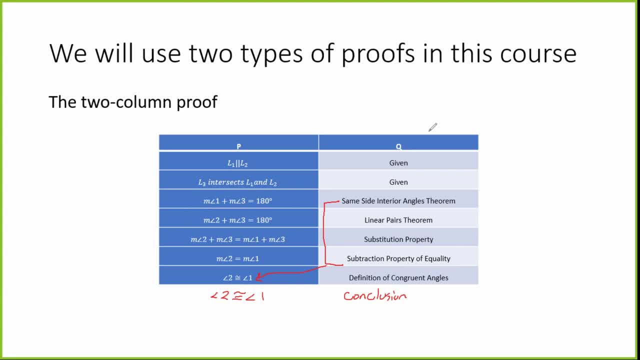 elegant end to your proof because you are saying we've accomplished what we set out to do and we've reached our conclusion or whatever came after then. one other thing you can do, and it only makes it easier to reference if you're getting more complicated. you can call this hypothesis one. 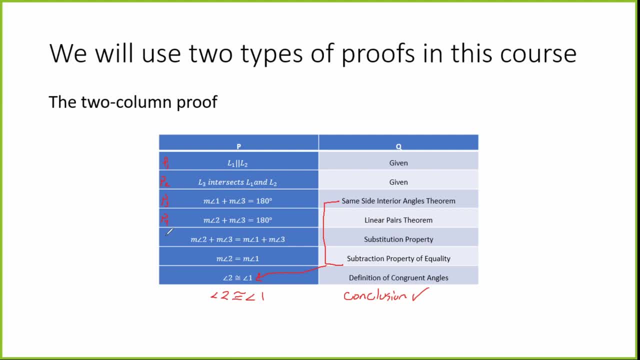 two, three. and the reason we can start calling these hypotheses is because something like this is already well known in math. right, we all know the substitution property, so we can say here that we can make substitutions based on these both being equal to 180. so really, it's not really telling you, you're doing it here. the nice thing about calling this hypothesis one. 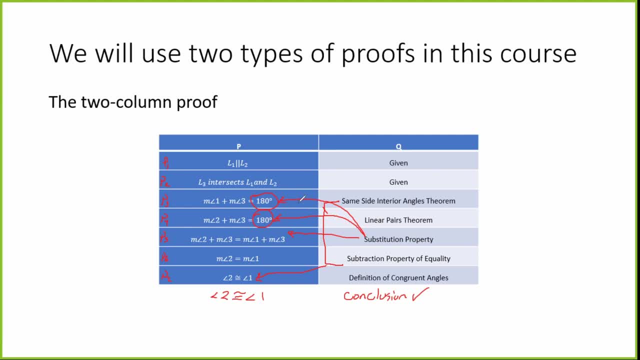 and two is that you can actually call back to what you're doing there. you don't have to do that either, but it does make for a more convincing paper, and if you're doing a more complex proof, it's actually easier to just reference back to, you know, p4 or, sorry, p5- to show that we did substitution and that. 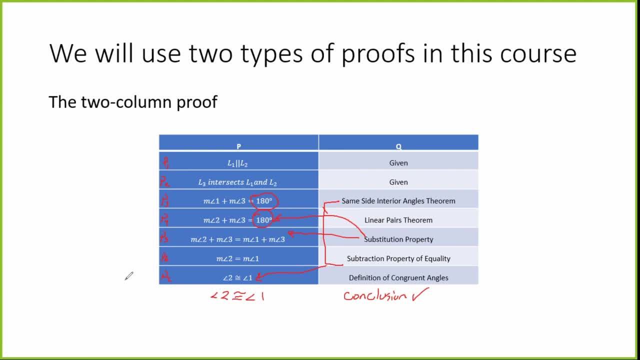 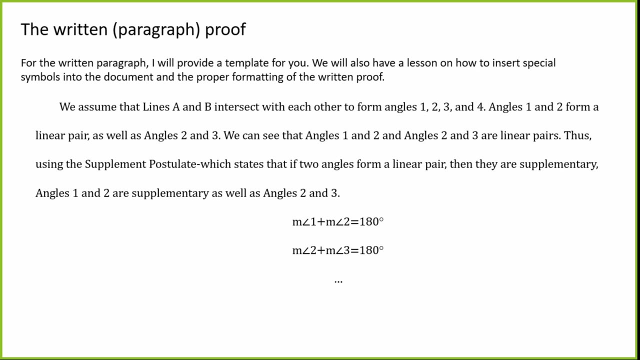 we're recalling that for another step. so the next style of proof that will briefly go over here is the reds and paragraph proof, and this is going to be necessary for your second writing assignment as well, and i will provide you a template to fill out. i will provide you. 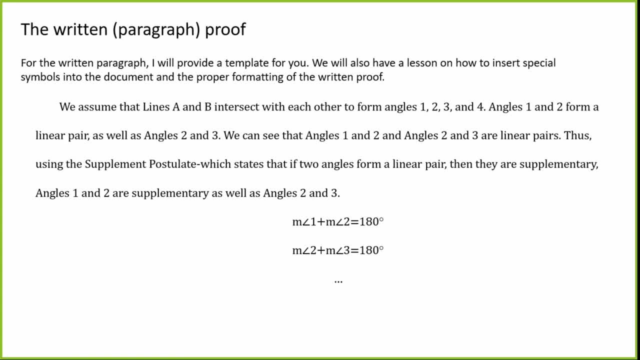 a list lesson on how to write all of our symbols mathematically so that you can have it look as it's supposed to be and formatted correctly. that's actually part of the rubric in quarter twos. writing assignment is that you've actually put the symbols in and you've made it look like a semi-professional paper. it's 10%. 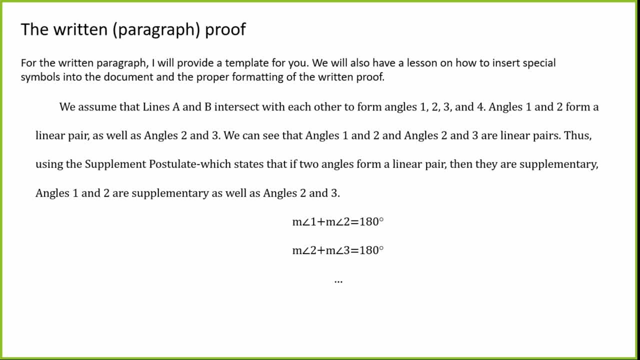 of your grade. so it's good to get this started today or as soon as possible, and I would like you guys to all practice it and I will make that available for you on Friday. that's part of your bonus problem set, okay, so one big thing, so in. 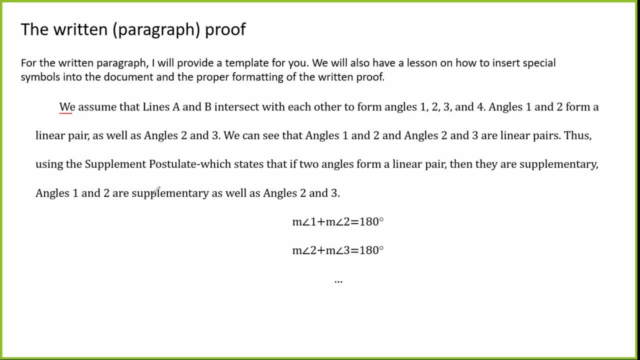 math, we. we never say I. you are not standing alone proving these. you're using countless other people's work, ideas, proofs. everyone that's been involved in this program has been able to use these, with the help of a lot of in your life, has gotten you to this point. so we credit everyone and we use the word we never i. 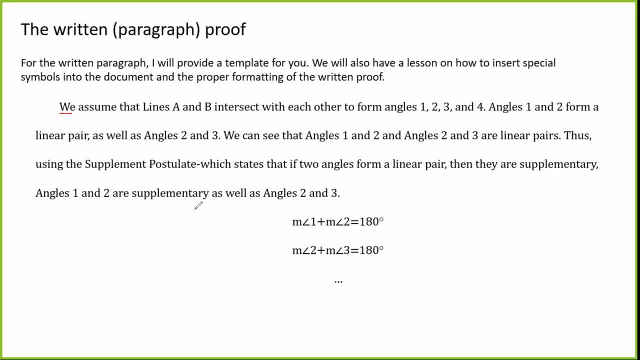 because i have not done any of this by myself. so we always start with: we assume. assume means we're looking at the hypothesis and whatever is given there in our picture or if, then statement, we're going to use that right now. so it says we assume that lines a and b intersect with each other to 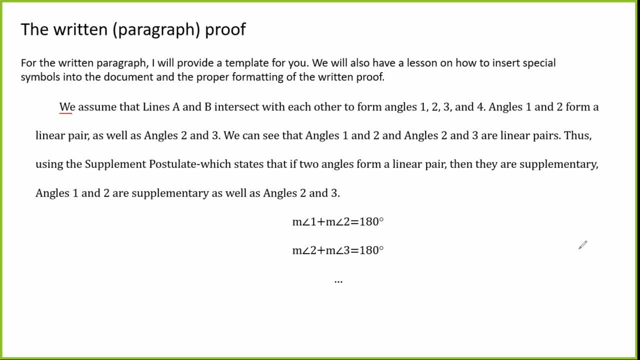 form angles one, two, three and four. so let's just kind of look at what that looks like. i'm already starting to have a suspicion here that we're looking at the vertical angles theorem. so here's line a, here's line b. let's label them. so again, line for l and that's line a. i'm going to double. 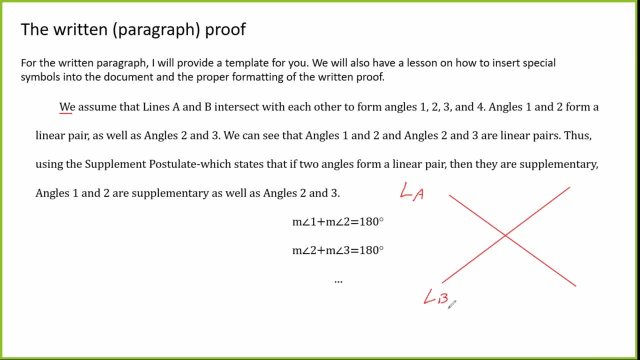 it up on that line. so let's go to this one and make that line b. don't want to double label a line and they intersect each other to form angles one, two, three and four. angles one and two form a linear pair, so i know that they have to be. 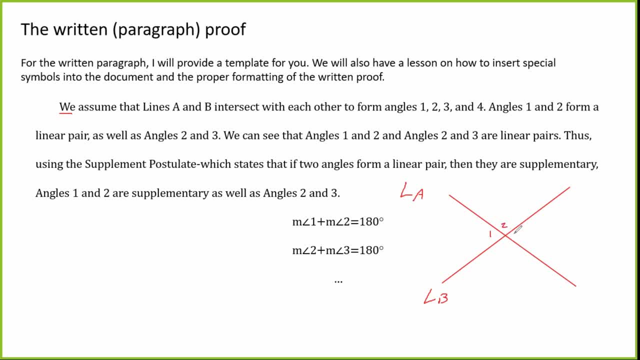 a linear pair, as well as angles two and three, and we can see that angles one and two and angles two and three are linear pairs. thus, we have thus using the supplement postulate, which states that if two angles form a linear pair, then they are supplementary. angles one and two are supplementary as well. 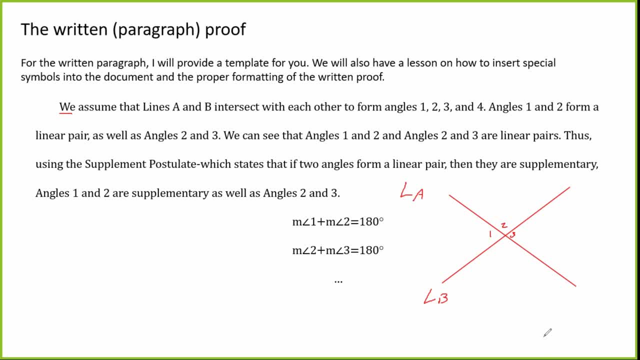 as angles two and three. this is a very beginner's proof, right? it's just saying that we are going to use linear pairs and what this is really doing is priming you to move into a vertical angles theorem proof. but let's see if what we have here is true, would the measure of angle one? 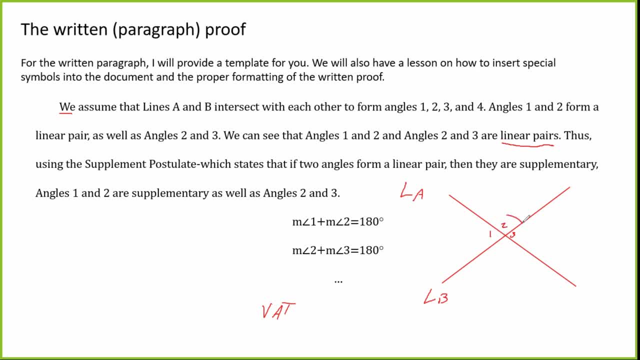 plus the measure of angle two equal 180 degrees. well, yeah, we know that they are a linear pair and by definition, so you can see that we explained that already. but now we have to show the math, and when we do that, we always make sure we center and only show the steps. if i needed to. 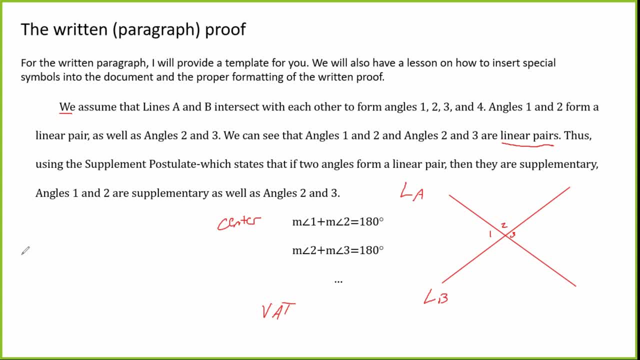 put another sentence in between these. i would go back over here to the left hand side, start a paragraph. all of your work that you did in your two column proof- and this is why i always start with the two column proof can be used- you go down your q side and you start with your givens. 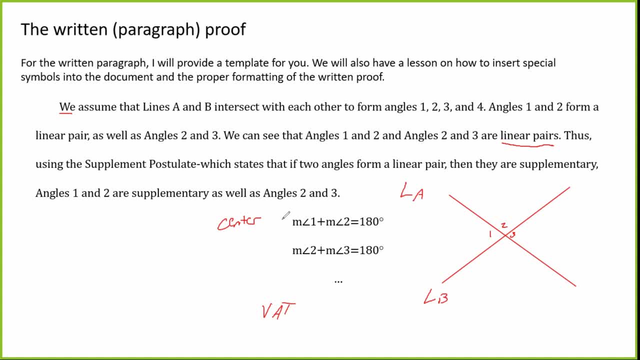 and each of your conclusions and as you do the the conclusions, you need to show the work from your hypothesis in what's called block formatting and that's where it's censored and stands alone. this is also why we always double space. does the measure of angle 2 plus the measure of 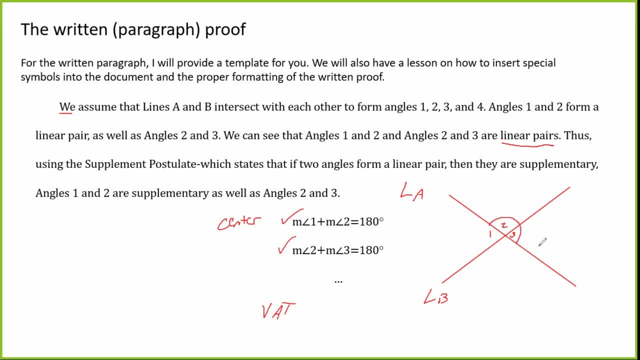 angle 3 add up to 180 for sure. now, let's say I wanted to do the vertical angles theorem. well, what I can say then is if the measure of angle 1 plus the measure of angle 2 is equal to 180, and the measure of angle 2 plus the measure of 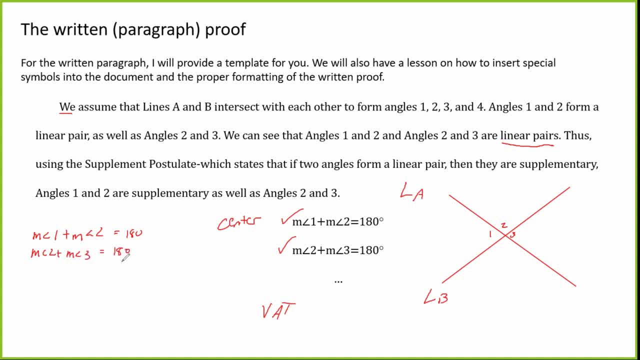 angle 3 is equal to 180. by substitution I can set the left-hand sides equal to each other and through the subtraction property of equality I am now left with the measure of angle 1 is equal to the measure of angle 1 plus the measure of angle 2 plus. 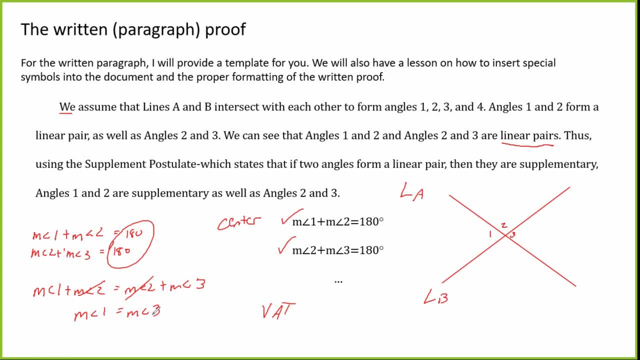 of angle 3, and that's what the vertical angle theorem tells us. this angle is congruent to this angle and this angle it's congruent to this angle, which we'll go ahead and label as angle 4. so if we wanted to, we can borrow, and this is why. 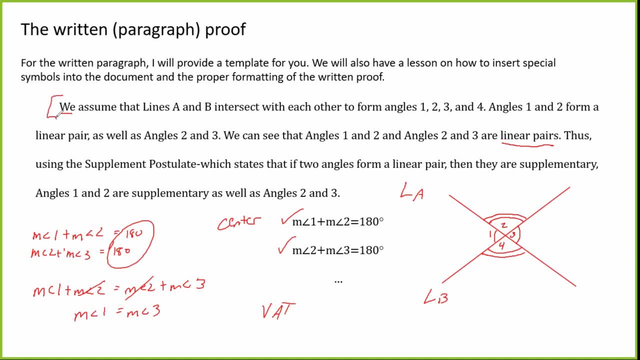 we don't say I, we say we. we can set up a vertical angles proof. almost exactly the same up to here. what we would then need to do is say something like: and we will show: angle 2 is congruent to angle 4 and that angle 1 is congruent to angle 3. 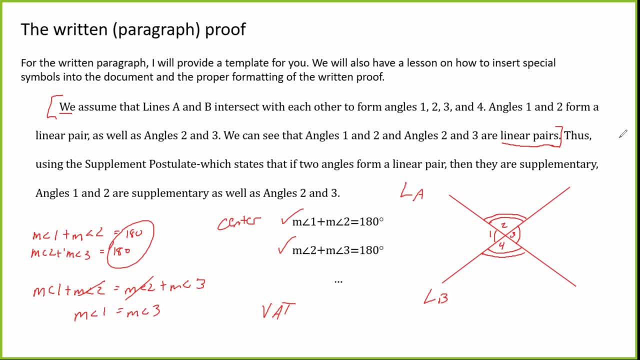 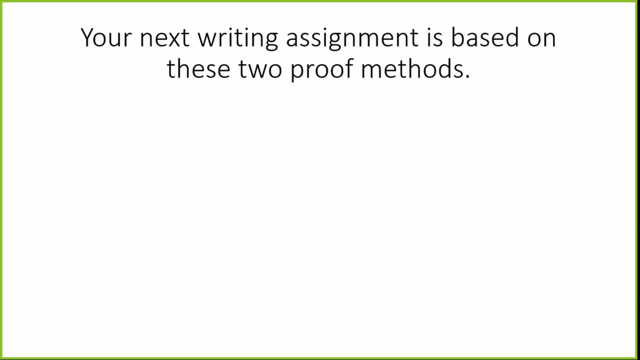 thus proving the vertical angles theorem. so this is really what this is all about: just putting everything we've kind of talked about, all of our reasoning skills, together and coming up with a full-on proof of it. you so, like I've said, your next writing assignment relies heavily on both of 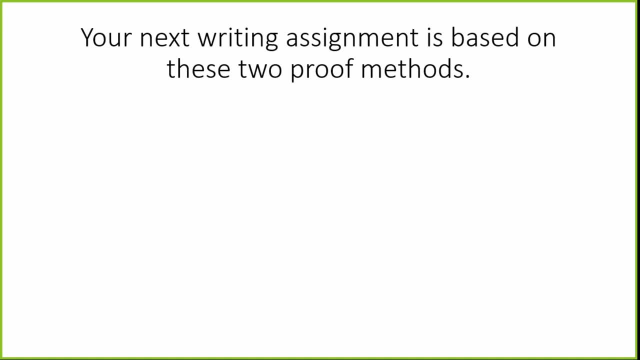 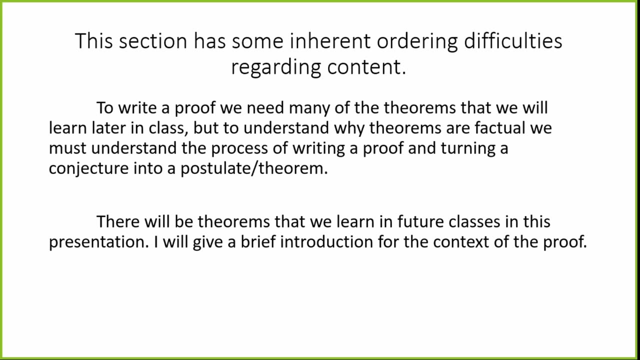 these styles of proofs. your homework are gonna look like this. fortunately, though, for the homework, you're gonna have a lot of drop-down menus with options, so use your prior knowledge to make educated inputs there, and we're gonna actually look at a couple of the homework problems at the end of this, but as I've 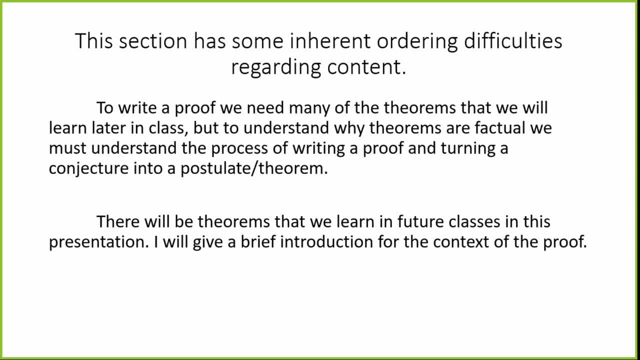 said in class and on the zoom meetings, this section does have some enhancements that you'll notice. in order to get started, hey, if you've got questions, feel free to take the time to write them down in the chat box and I'll answer them for you as we head into the next section. I'll be Nosy with the whole. 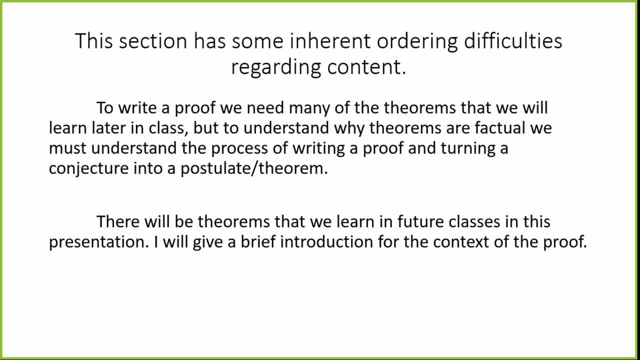 trick or two. I'll be Nosy with the next section of the class and I'll be talking about not only the basic concepts of basic concepts, but how to prepare for the next section, and I'll be having a little moment to come back to play with my other components of basic concepts that we'll be speaking. 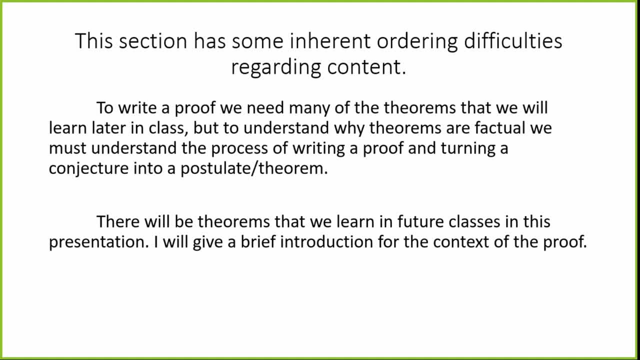 about in the next session. if you want to know more about our next section of online training and the things related to the сrm, I said in the last section that I'll be sharing with you soon about our upcoming courses so that you can get a chance to learn more about some of these components that we're going to be. 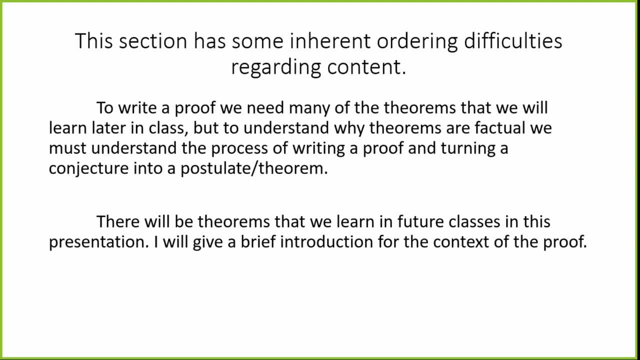 talking about in our next session. I'll be talking about some of these things that we've forward. the things I'm going to show you are really rely are going to be heavily relied on during quarter. I mean section two of our class and I'm pretty sure the 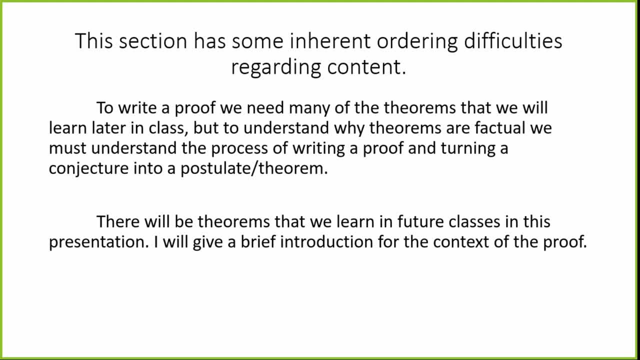 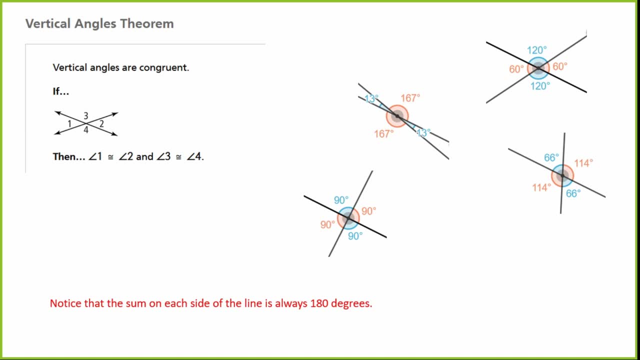 first one up is the vertical angles theorem, but most of our classes going forward are going to be introducing a couple theorems and then showing examples of how they work, working with them and then moving on. so up first we have the vertical angles theorem and with that I like to think of this kind of 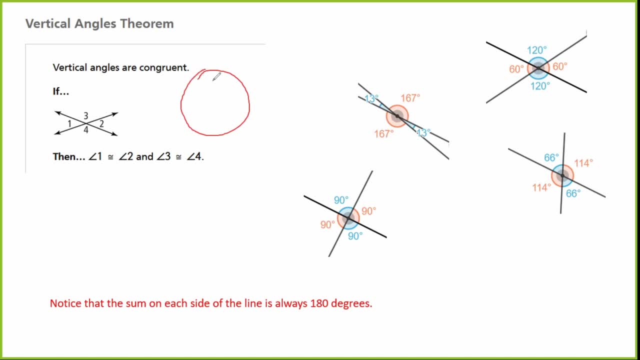 as the hands-on o'clock. if I were at 12 oh five, I can imagine that these are extended and then this one and this one are equal, and then this one and this one are equal. overshot that, that's pretty much what it's showing you here. these are. 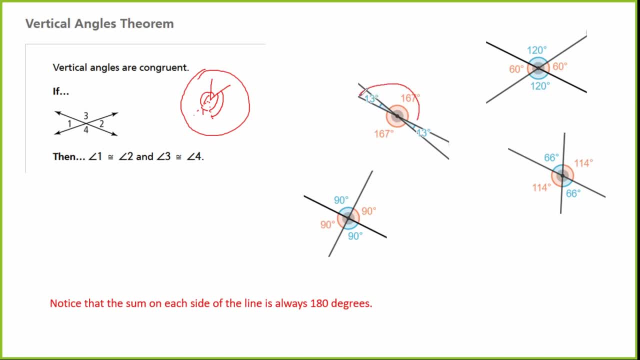 all the same things. so I'm going to show you the vertical angles theorem. and then the vertical angles theorem just makes linear pairs and it tells you that on each side of a line, so on each side of line one, if I have 167 here, I have to. 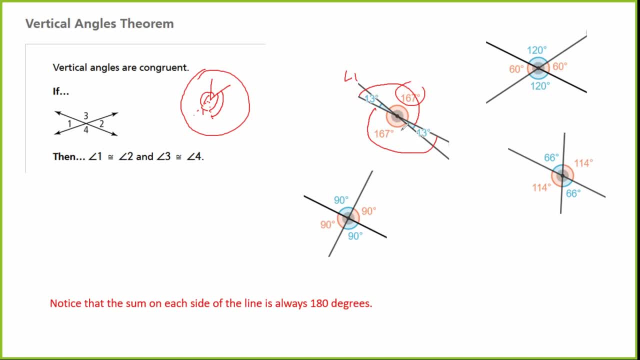 have 13, and if I have 13 on that side with 167 on the opposite side of the line, I have the exact same thing. if I were to look at line two now my 13 associates here and then I have it again here and you can see in the diagram that they're color-coded for us. so it's a. 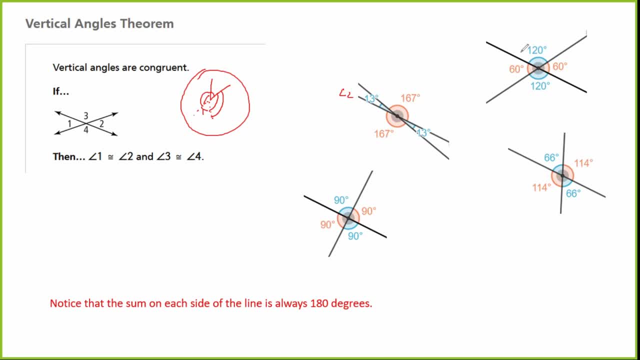 little harder to see that. but here's another good. this is a one of the more regularly used linear pairs: 120 degrees. right, that's my obtuse angle. here's my obtuse angle. see that they have the same value by the vertical angles theorem. and then my two acute angles by the vertical angles theorem are also the same and 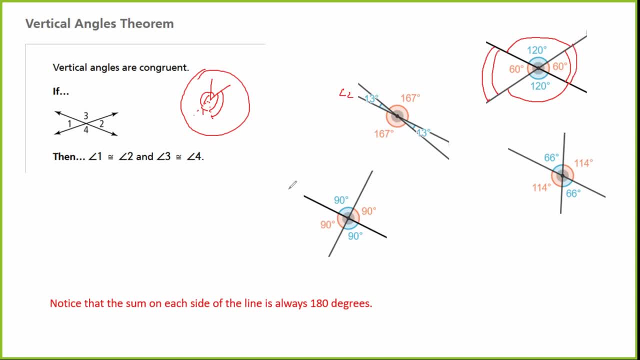 this kind of makes sense. think of this as if this is a one-sided integral, and I'm going to show you how to do that. so these are two pencils and you put them together as a T. as you rotate the pencils without moving the center points, the angle changes, but its opposite side changer at. 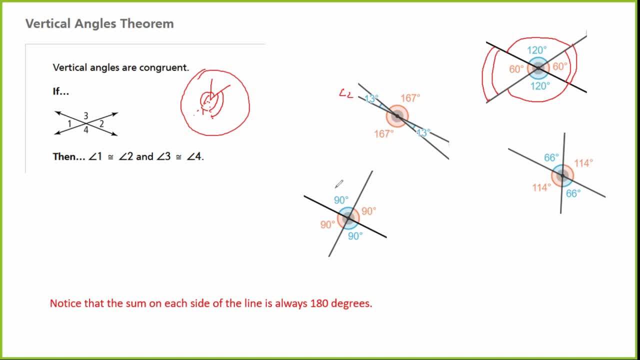 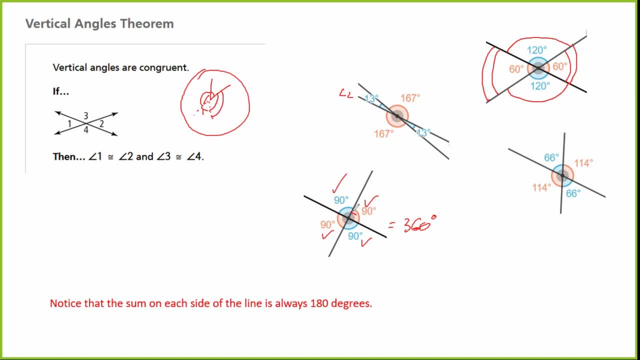 why these are designed that way. we could also draw here our perpendicular symbol and by the vertical angles theorem, if this one's 90 degrees, then this one's 90 degrees. and by our linear pairs theorem, this one must be 90 degrees, so that these two add up to 180, and these two must add up to 180, so we can also end up. 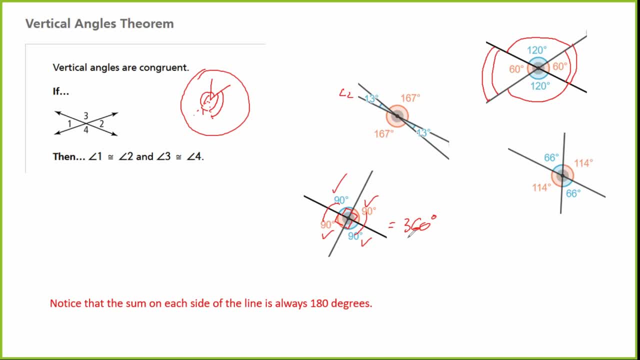 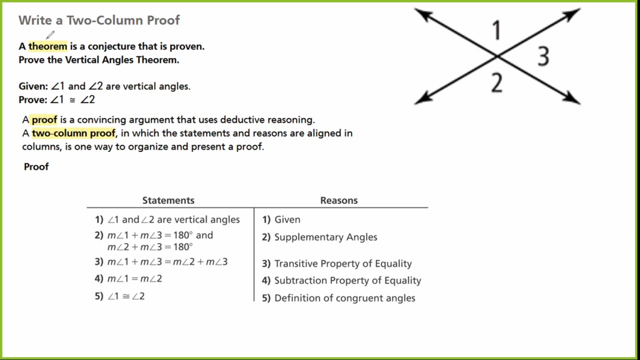 with a square on the inside and the interior angles of a square also sum up to 180 degrees. so let's look at a two-column proof for this. so again, a theorem is a conjecture. that is just proven. so now we can start doing proofs here. you can go back to the previous slides and start writing proofs from: 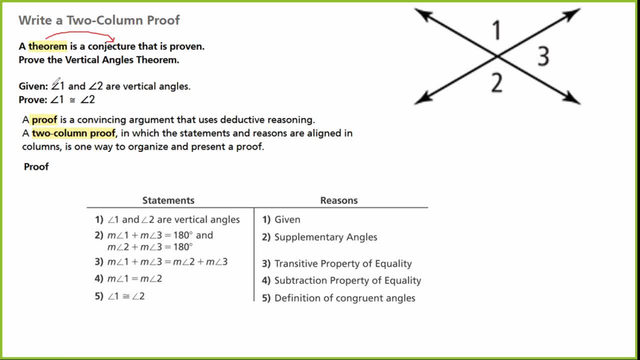 those. but let's see, given okay, we're going to use the vertical angles theorem to prove that two things are true, that angles are true, that two things are true, that two things are true, that angles are true, that two things are true, that two things are true, that 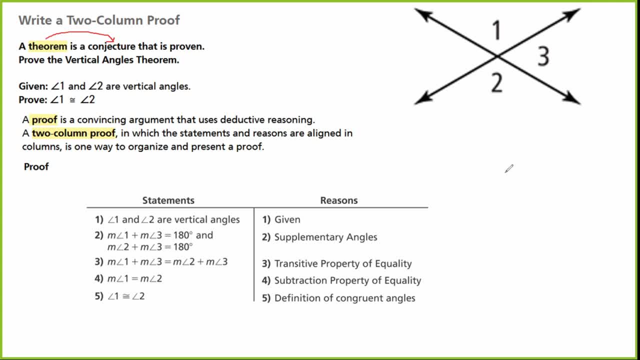 one and angle two are vertical angles. now, they were kind of nice to you here and they actually associated these vertically with each other. but just because the English definition of vertical means up and down doesn't do quite enough for our math class to prove it. but here's how we can do it, so it 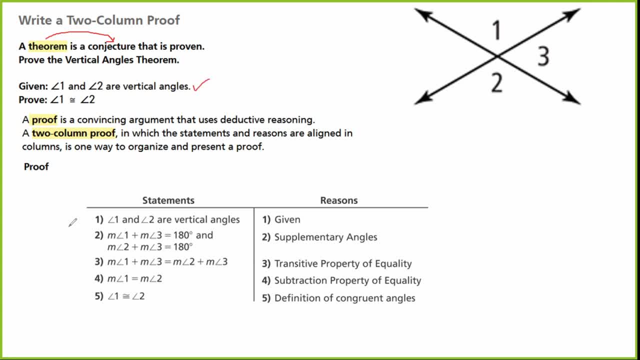 says: given one and two are vertical angles. so notice that the first step here is that angle one and angle two are vertical angles and that's our given perfect so statements. we won't write that. we're gonna write P and Q. the measure of angle one plus the measure of angle three is 180 degrees and the 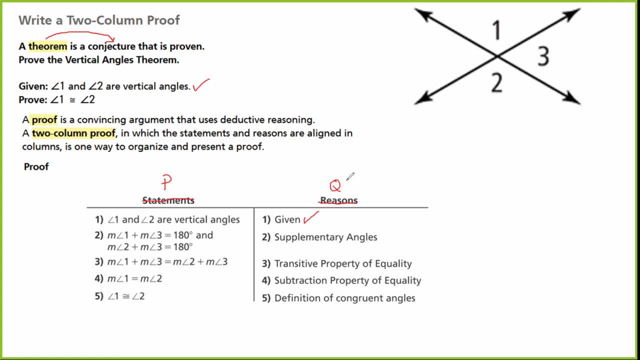 measure of angle two plus the measure of angle three is 180 degrees, and they're saying that's by the supplementary angle theorem. what else could we call that? well, one in three, and two and three, or we could write the linear pairs and would add up to 180. so again, two different answers that mean exactly the. 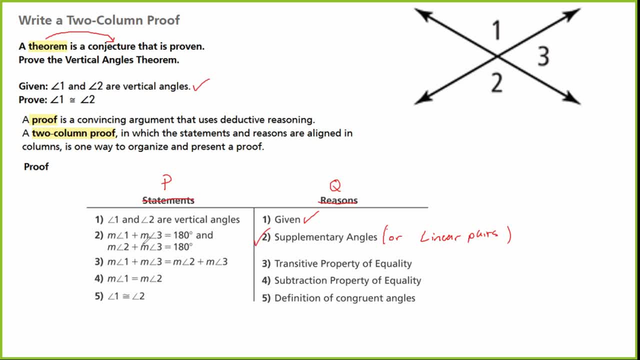 same thing, so we do have more freedom in this class, but now we need to verify that that's true before we move on. one and three are in fact linear pairs and would add up to 180. two and three would also add up to 180, and then again. 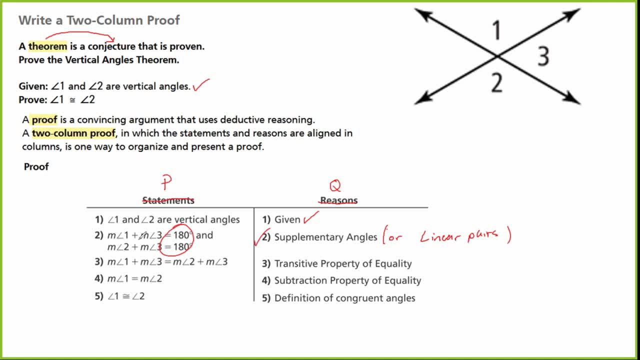 because they both equal 180. we can set the left-hand side of both of these by the transitive property of equality, or substitution would be another way right, because you can substitute the value for 180 for this, or you can substitute that for 180 there. so again, 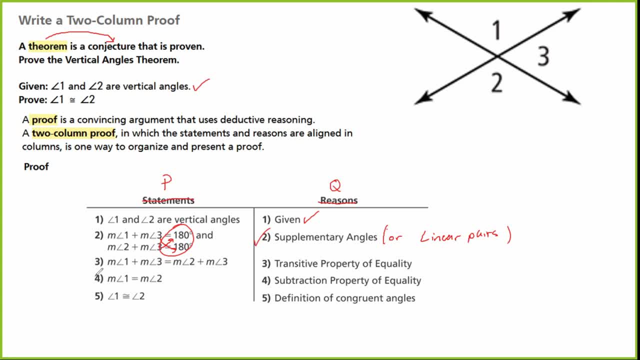 another option, and we show that that's true by the subtraction property of equality. we can get rid of both of angle threes and we've done everything we've set out to do. the only thing that I said sometimes you could start would be P 6. 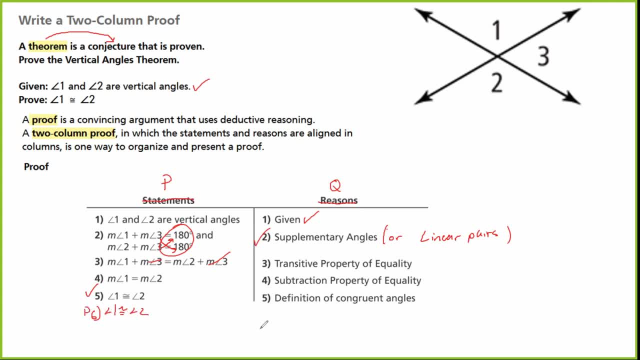 and just show that Q 6 is conclusion. again, you don't have to do this. there will be some professor some time in your life going forward that potentially will, so I want to keep that at least available to you. alright, let's look at another theorem. and of course, you guys. 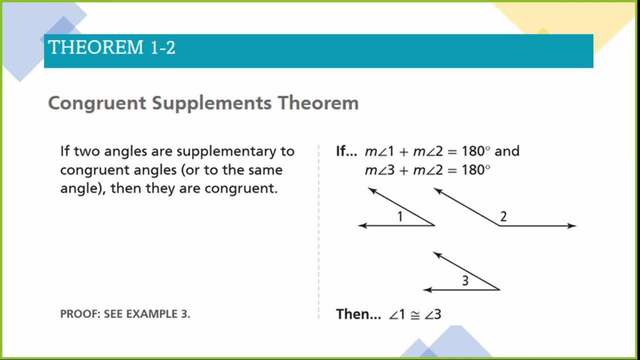 can pause this, since it's on a video and you have time to copy it down. congruent supplements theorem just tells us that if two angles are supplementary to congruent angles, or that's just all we need to know- in order to compute the solution, we need to be able to compute the solution. we need to be able to compute the. solution. we need to be able to compute the solution if we already know that we need to be able to. of course, if we only have 30 numbers of the right, one square is equal to 50. we need to be able to multiply: 50 plus 520 is equal to 50 plus 580 is equal to 50?. 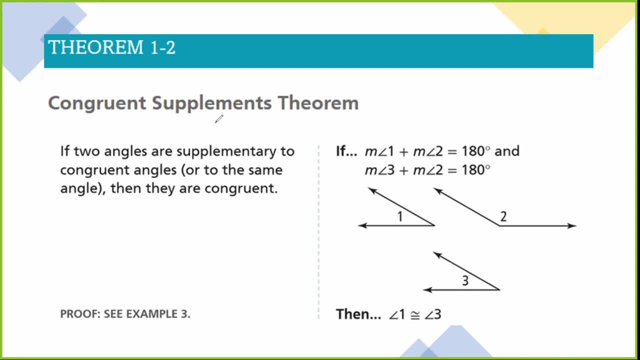 to the same angle, then they are congruent, and what? so? that's a pretty confusing way to look at it. what it's saying here is: if the measure of angle 1 plus the measure of angle 2 equals 180, so if I were to move this one over? so 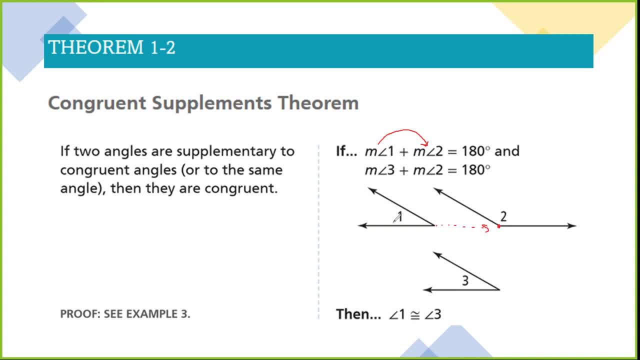 that their vertices were matched, I would have a straight line. what it's saying is that I can then move angle 1 out and slide angle 3 so that their vertices are matched. and I would also have a straight line because both angle 1 plus angle 2 is equal to 180 and angle 3 plus angle 2 is equal to 180. I can say the 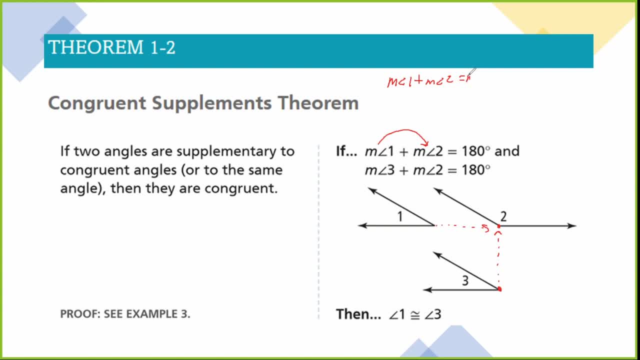 measure of angle 1 plus the measure of angle 2 is equal to the measure of angle 3 plus the measure of angle 2, and by the subtraction property of equality, I am left with the statement: the measure of angle 1 is equal to the measure of angle. 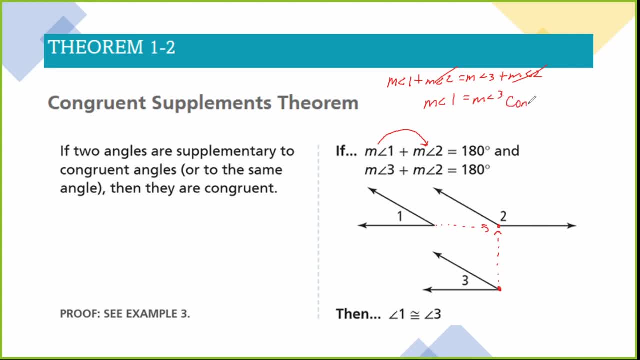 3 and that is our conclusion. so right there, I can take what's on our screen and make that a two-column proof, and then I can turn that two-column proof into a written paragraph proof. wouldn't be much of a paragraph, only take two sentences other than the setup. 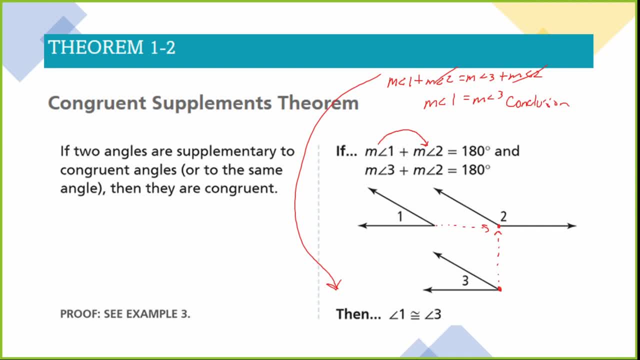 in the closing, but that's exactly how we do that. our next theorem is the congruent complements. so let's talk about the difference between supplements and complements. supplements means adds to 180 degrees. notice when I move these into the position: they complete a straight line and add up to 180 degrees. what 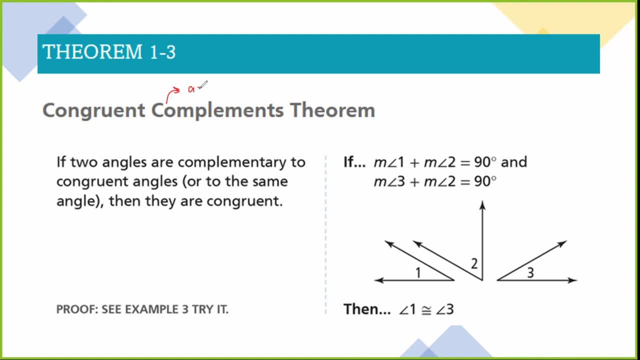 complements means is that they add to 90 degrees. so if two angles are complementary, so Lenovo thinks that they add to 90 degrees. so again, if i take two angles and when I put them together, so if I move angle 1 to here, so that their vertices touch and that these Rays, or directly on top of 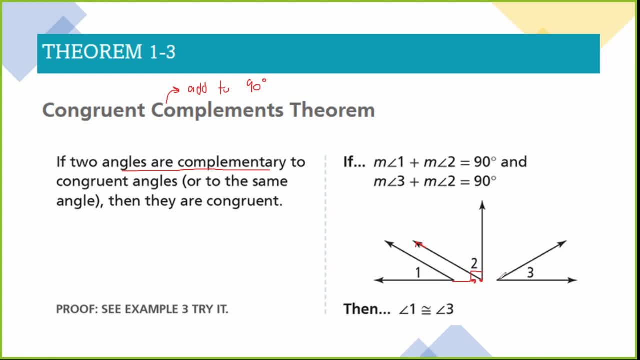 one another. if i get 90 degrees out of that and then I can flip three over, associate it so that it's in the same fashion as I ngle one and slide angle 3 and it also gives me 90 degrees, then angle one is equal to angle three, basically what this is. 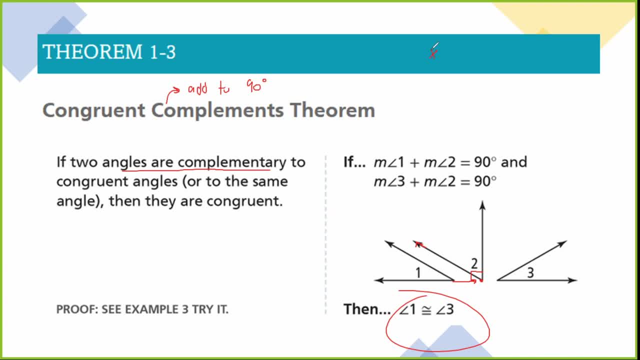 telling you algebraically, since we're kind of fresh into geometry, if that, if x plus y is equal to z, all right, let me apologize for the jump there. i chose to use a greek letter for this example and realize that might be a little bit too much here. 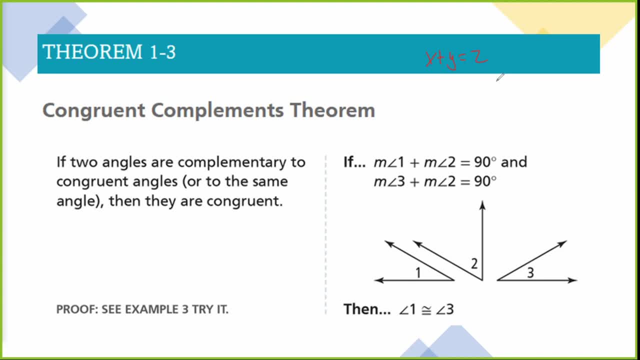 so let's go back to if x plus y equals z and a plus y equals z, then i can say: since these two on the left hand side are both equal to z, they are equal to each other, and i can subtract out my y's and i get x is equal to x. of course x is equal to x, but x is equal to a, and that's pretty much. 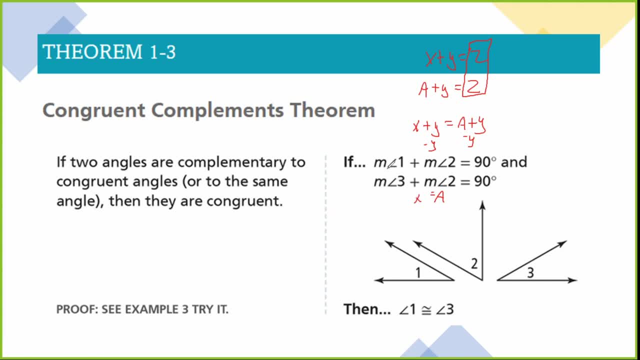 what we're doing here. so, except for now, instead of our variables being one character, there are three characters here, but they're still variables nonetheless. these are stand-ins for whatever measure of angle one is. so let's look at this if it were to be um numbers. let's say that the measure of angle one 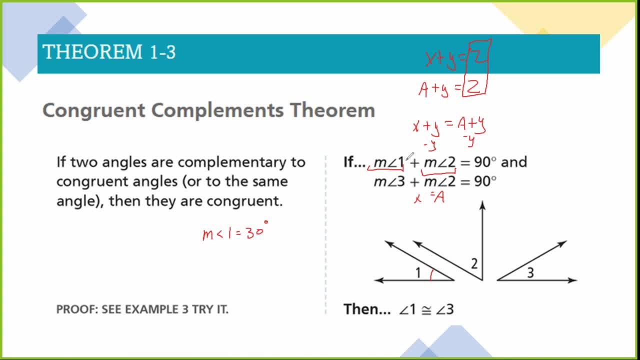 is 30 degrees. well, for measure of angle one plus the measure of angle two to equal 90, i can say that 30 plus the measure of angle 2 is equal to 90 and get the measure of angle 2 is equal to 60.. 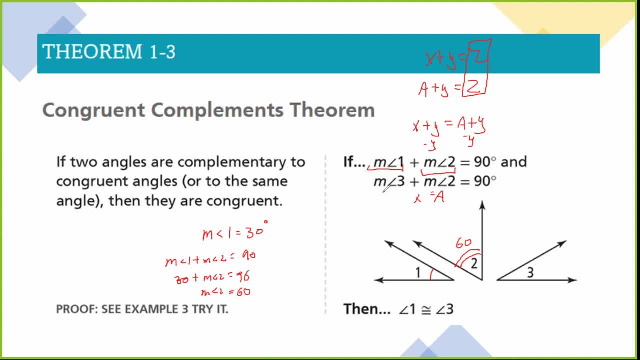 but now that i know this is 60, this also must be 30, and it shows that these are in fact congruent. so that is our congruent complement theorem. a lot of this stuff is things that you've learned in late elementary school, early middle school. 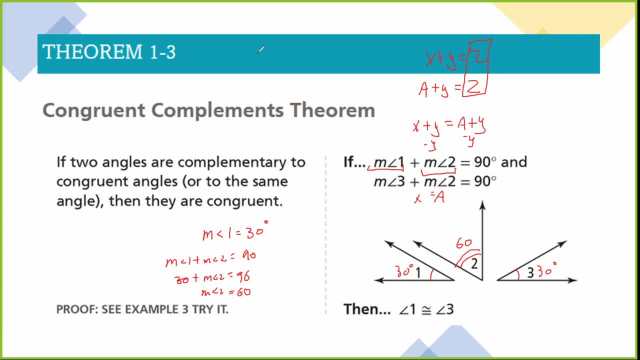 and when you ask: what are you going to use this for in the future? the answer is this moment, right here and showing that complementary angles add up to 90 and supplementary angles add up to 180. up next, we have our first theorem with no name. it's called theorem 1, 4. i believe might be 1, 3, no. 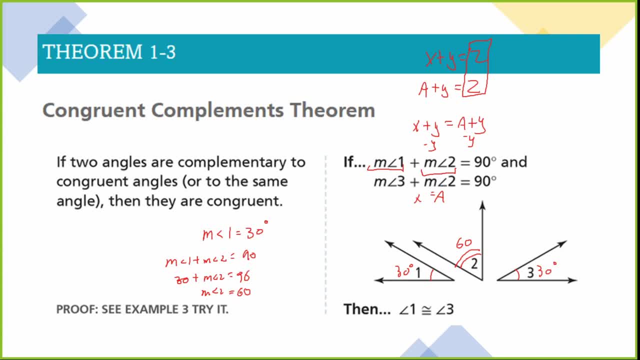 it's 1- 3 is on the screen, so 1- 4, and this is not given a name because it's a pretty common sense one. so i'm going to flip over to that right now and go ahead and do that, and then we're going to do that. 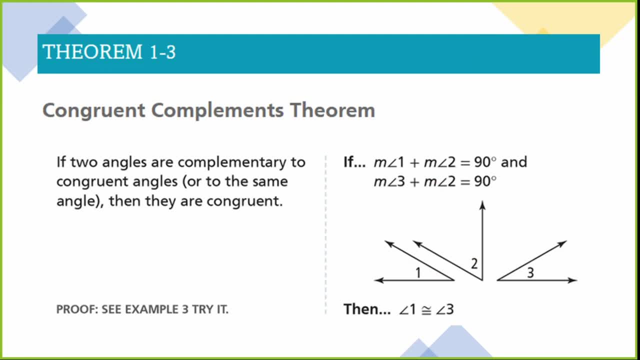 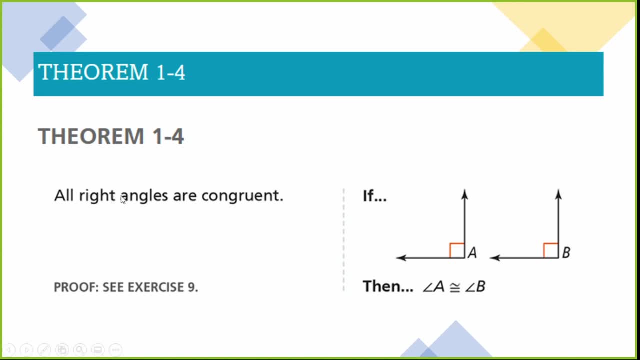 give you a minute to copy it down, all right. so one four basically says: all right angles are congruent. the definition of a right angle is that it is 90 degrees where at the vertex. so if the definition of something is that it's 90 degrees, then of course all right angles are. 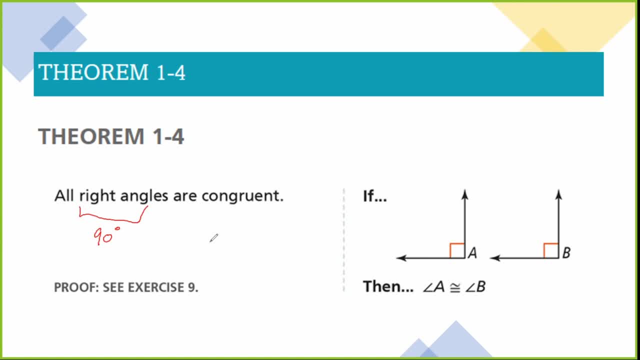 congruent. it's going to be a tough day on a proof if you are stuck, and that is something that you need to tell everyone, but it is. this is more of a just. it's good to know that all right angles are congruent to each other. anytime you see this, this, this or this, those are all 90 degrees. 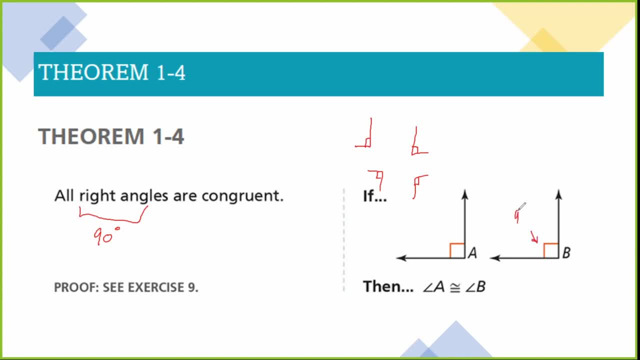 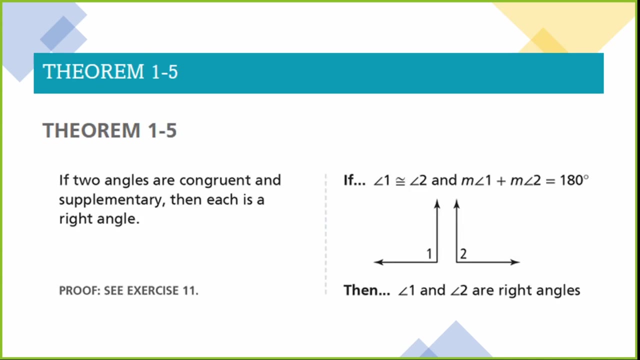 they're all equal to each other. this box again means 90 degrees. so that is theorem one four. we can call it the right angles congruency theorem, but it takes longer to say that than it does to make sense of it there in one five. if two angles are congruent and supplementary, then each is a. 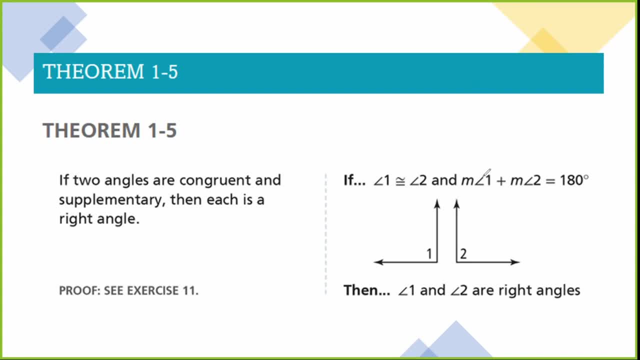 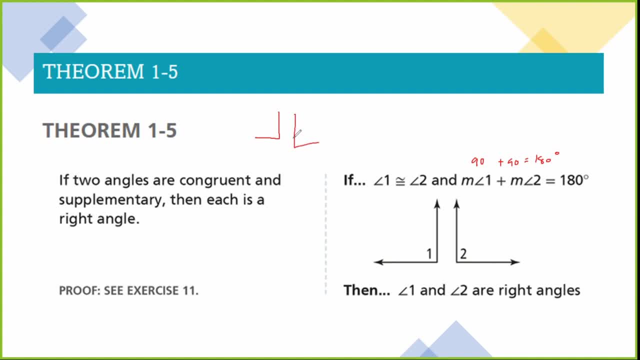 hypothesis correctly. so here's one, here's angle one, here's angle two, if they're congruent, then, and supplementary so if I add them together. the only way that can happen- let's do it visually really quick- is if I combine them, and then I can see that. 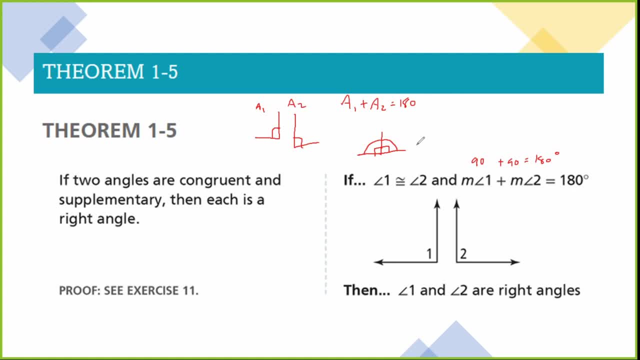 they make a straight line. so if they're on 1, 5, again it's a pretty obvious theorem to look at. if two angles are the same measure and they add together to make a straight line, well, I know they're the same and I know their sum is 180. I. 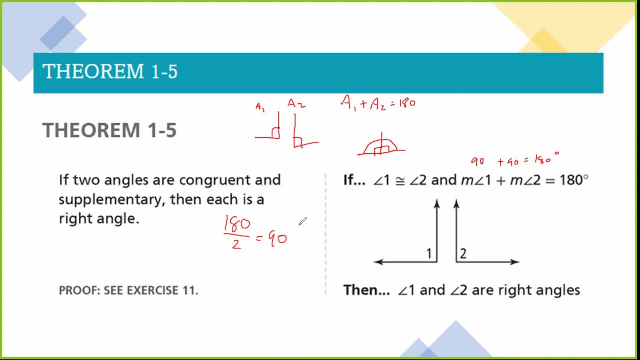 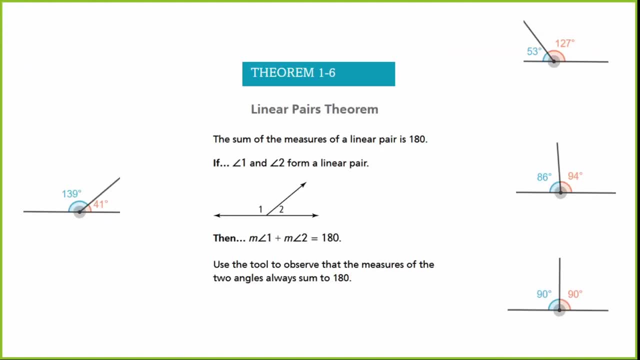 can just divide it by 2. both must be 90 degrees, all right, so we're gonna knock out a lot of theorems. today. we have our linear pairs theorem. let's formalize it. this is our sixth theorem on the screen and we've already talked about this one. 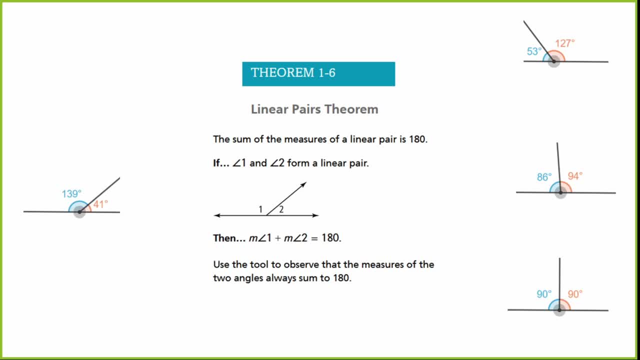 we just know that we have a straight line and an angle or array that bisects it. no, no, you can't say bisects, that's later on you'll learn what that means. intersects it or intercepts it, whichever way you want to look at that word. the 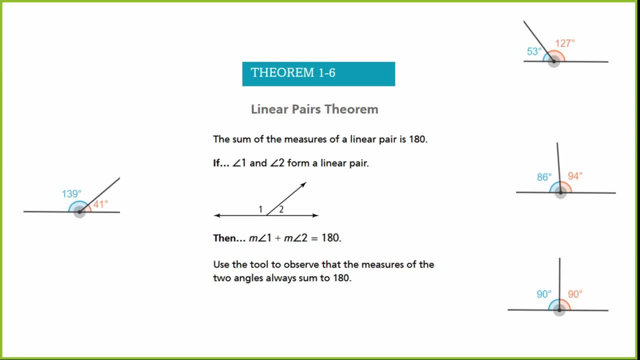 sum of those two angles is always going to be you 180 degrees. got a few examples up here: 139 plus 41 gives me 180, 90 and 90. this is 180. this also shows us that all right angles are congruent and congruent. 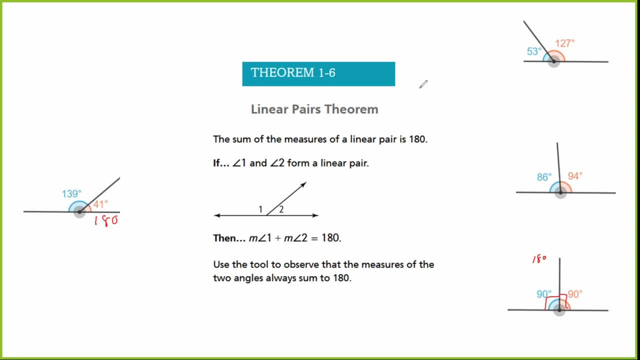 supplements must be 90 degrees, 86, 94. takes one extra step mentally to add the 6 and the 4, to turn that into a hundred, you get 180 and 53 plus 20, 27 is 80 and with that extra hundred tacked on on the front, there we again. 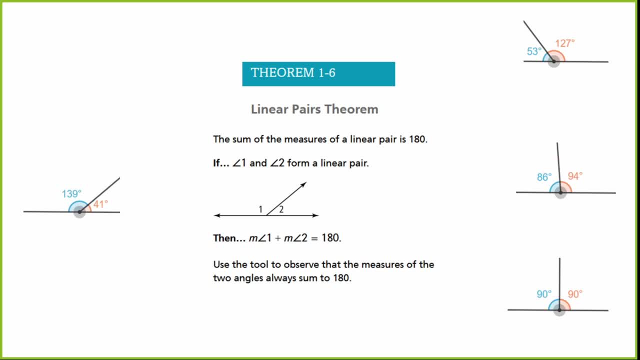 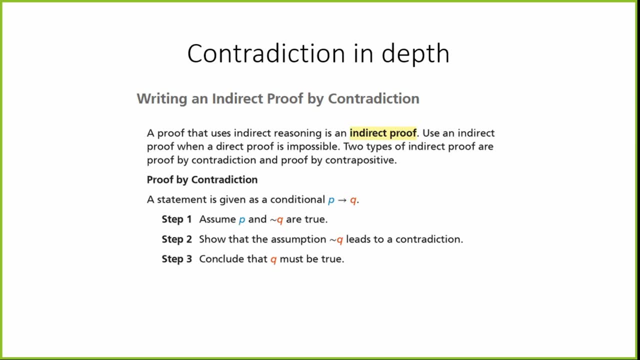 have 180 degrees. now we're going to move on to talking about contradictions. indirect proof is where you say if something, but if then? but we're going to assume that then is not going to happen. we're going to show it's actually going to happen and we're going to show that the assumption has led to a. 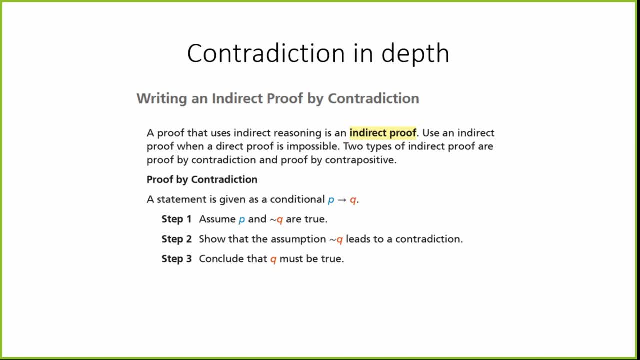 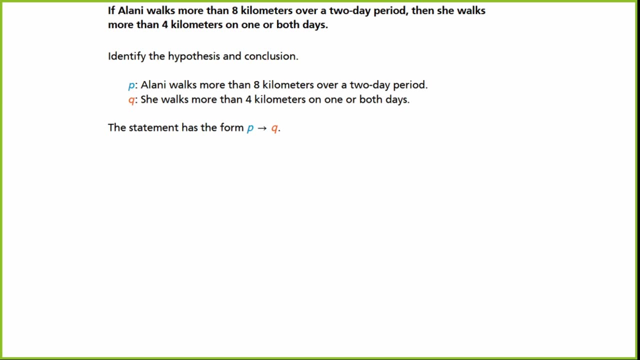 contradiction and then that it's going to conclude that Q 1 is going to be a あるタイプと正確な依頼 must be true. this one is best done by just looking at a problem here, and that problem is: if Alani walks more than eight kilometers, so we have our F. so 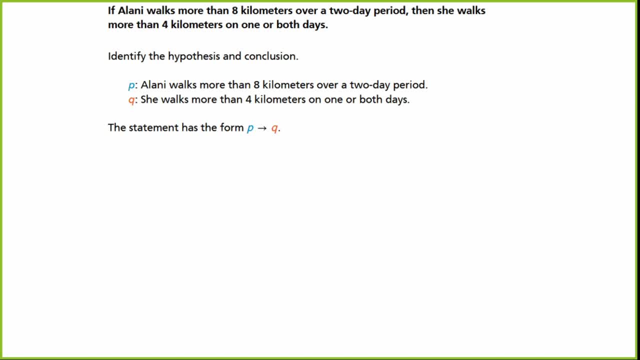 let's go ahead and color code. this, Lou's been our hypothesis, so let's get back to that. if Alani walks or than eight kilometers over a two-day period, and then in our conclusion, is green. if Alani walks more than eight kilometers over a two-day period, and then in our conclusion, is green. now that we're gonna get that same thing over here. if Alani walks more than eight kilometers over a two-day period, and then in our conclusion, is green. 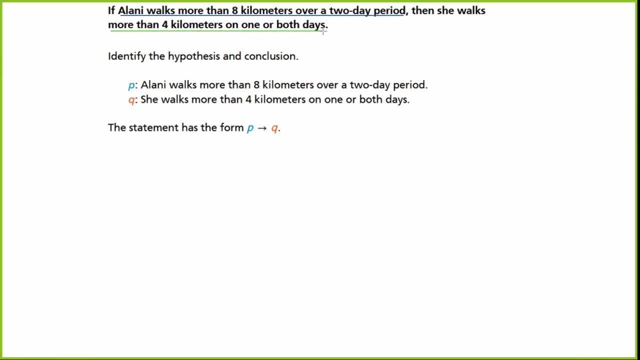 then she walks more than four kilometers on one or both days. So let's think about what that means algebraically really quick. So our P is: oh, let's not do that in green, That would be confusing. Our P becomes: well, let's do it on this slide here. 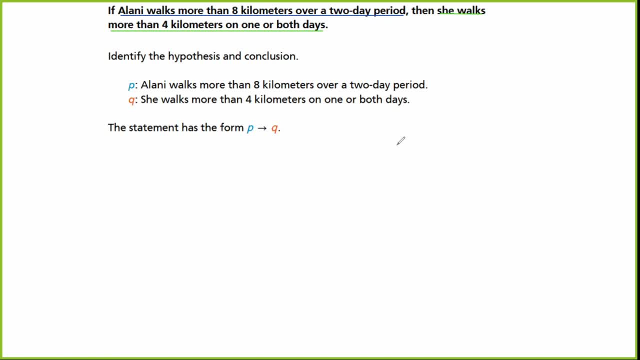 So first we're going to identify the hypothesis and the conclusion which we've done. Our hypothesis is: Alani walks more than eight kilometers over a two-day period And our conclusion is: she walks more than four kilometers on one or both days, And the statement does follow: the P implies Q format. 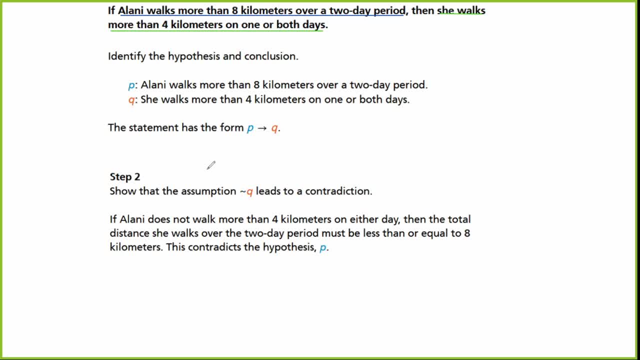 So step two is: let's show that the assumption- not Q, right, Remember, we read this word here as not Q- leads to a contradiction. So look how we have to change. All right, let's look at it and then we'll look at how we have to change it. 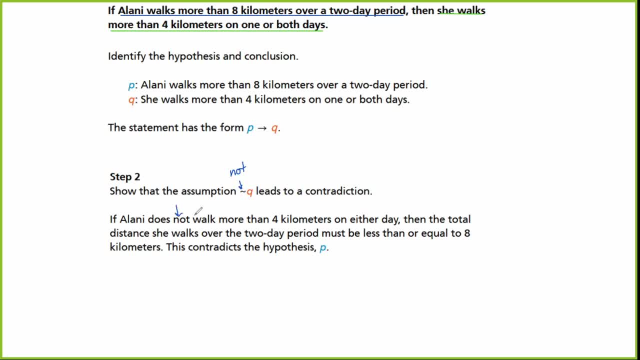 If Alani does not walk more than four kilometers on either day, then the total distance she walks over the two-day period must be less than, or equal to, eight kilometers, And this contradicts our hypothesis. So now let's go back through it and look at it algebraically. 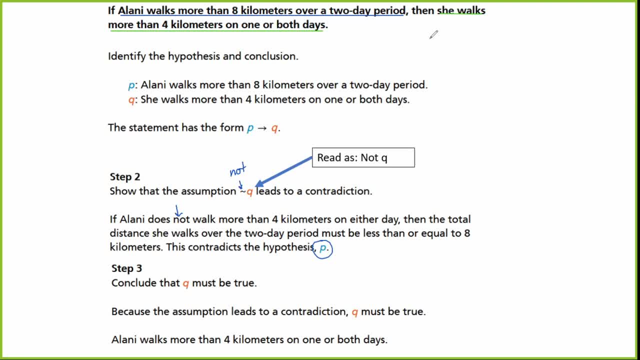 So if Alani walks more than eight kilometers over a two-day period, so two times D, right, two days- is greater than eight kilometers. Our hypothesis is that on day one she walks more than four And on day two she walks more than four, on one or both days. 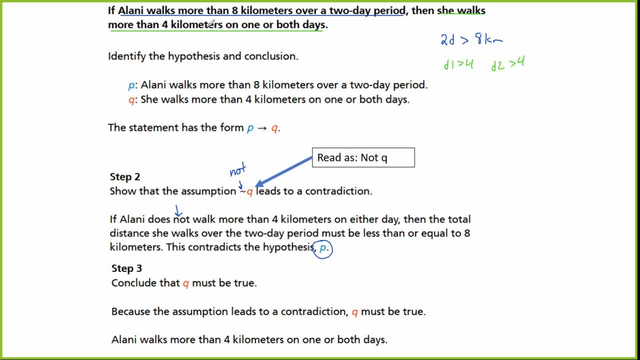 So both days has to be at least greater than four. So let's assume this is not true. Let's say that day one Is equal to four And day two is equal to four kilometers walked Well, Would her two days then be greater than four plus four? 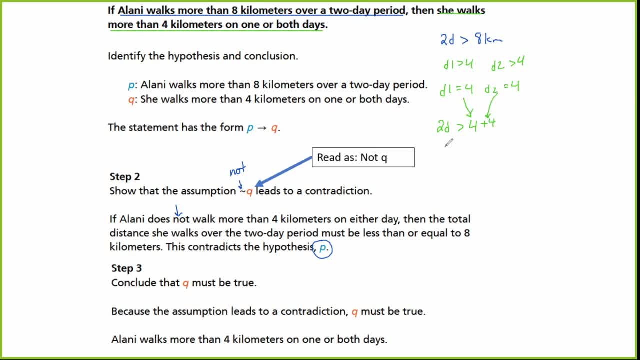 Right, here's day one, Here's day two, And in two days she needs to walk. eight, Is eight greater than eight? No, And this is a contradiction. What if I did less than four? right, I can pick any number less than four. 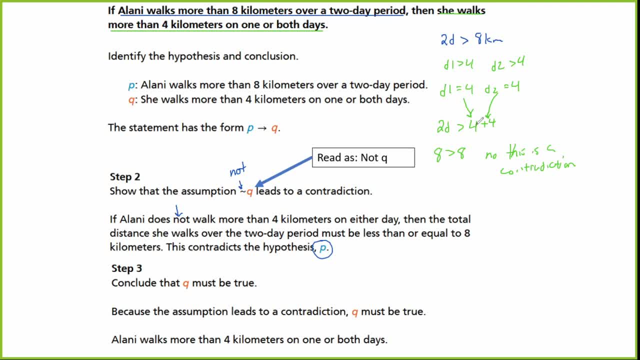 Well then we can see right away. if she walked three kilometers on day one, Let's erase that. Well, let's just do it down here. So now she needs to walk more than eight in two days, And she has three plus four. 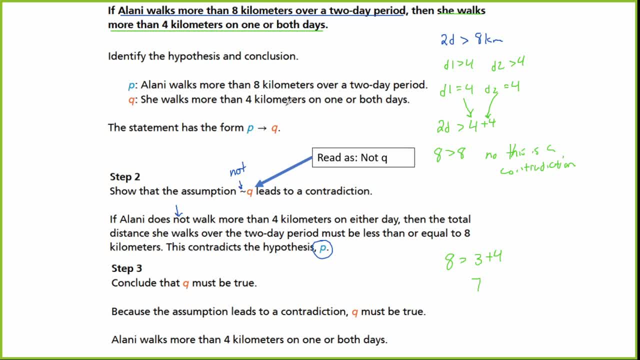 And that gives us seven. So now you're going to. I'd probably say: well, what if we just said she did ten kilometers on one day? Well then, we have to go back and consider that we have to negate this conclusion. 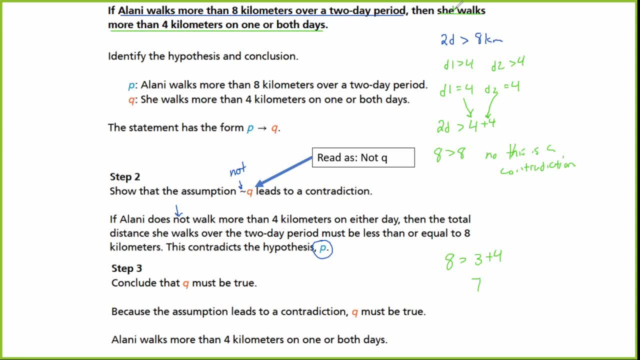 She Does not walk More than four kilometers on one or both days. So We have to keep it under four for both days, And that's what we've done here. We have day one at three, We have day two at four, for a total of seven. 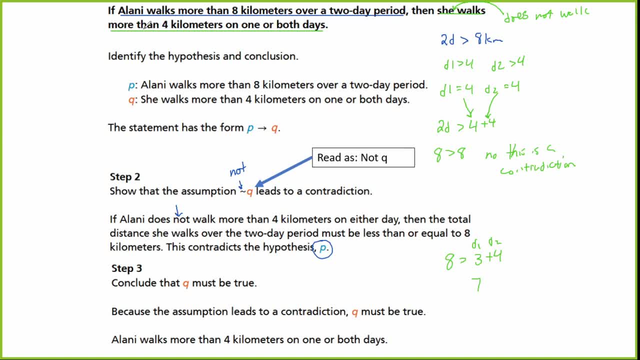 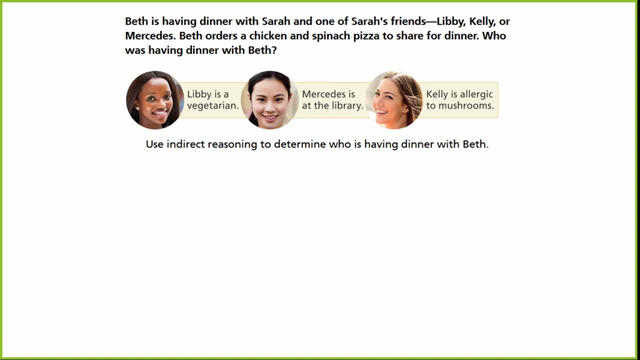 So we've now run into a contradiction here. She must walk more than four kilometers on one or both days for this to be true. All right, So let's look at a word problem that's basically and strictly English, right? There's not too much math involved with this one. 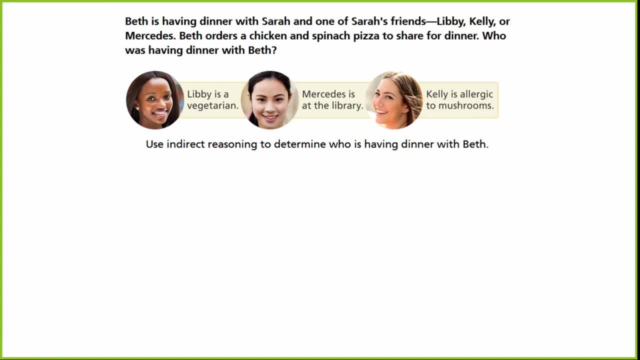 But we're going to use our reasoning here To try and figure out who Beth is having dinner with. So let's read the problem. Beth is having dinner with Sarah, and one of Sarah's friends, Libby, Kelly or Mercedes, Beth orders a chicken and spinach pizza to share for dinner. 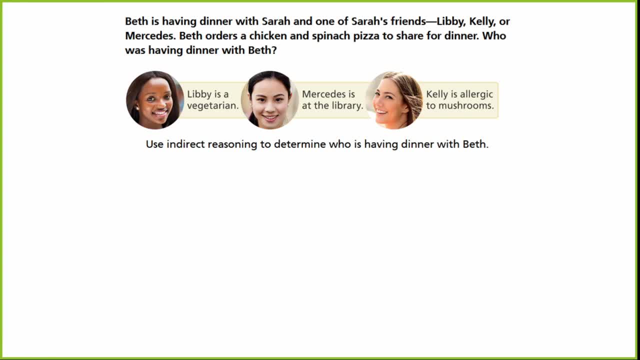 Who is having dinner with Beth. So we got to look at a couple of things here. Libby is a vegetarian, Mercedes is at the library And Kelly is allergic to mushrooms. So now we're using our indirect reasoning To determine who is having dinner with Beth. 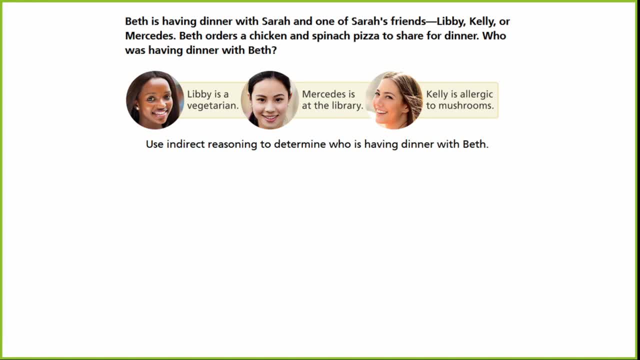 So the best way to look at this in a mathematical sense That I've tried to prime you with in the previous slides Is: do any of these set up for a contradiction? Oh, Beth is having dinner with Sarah, So that's definitely a go for. 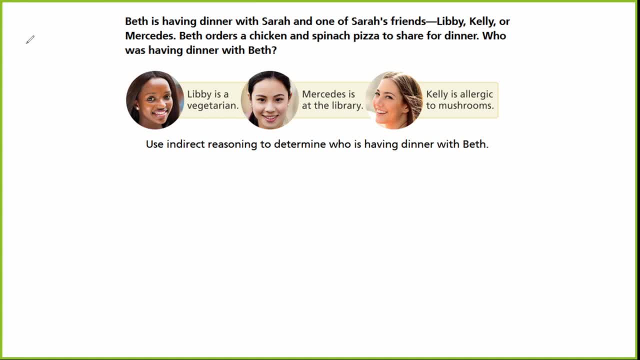 Let's fill out our hypothesis first, Or let's look at our givens. Beth is going to be at dinner, Sarah is going to be at dinner, But which of Sarah's friends will be there? Well, Let's look at the outcome here. 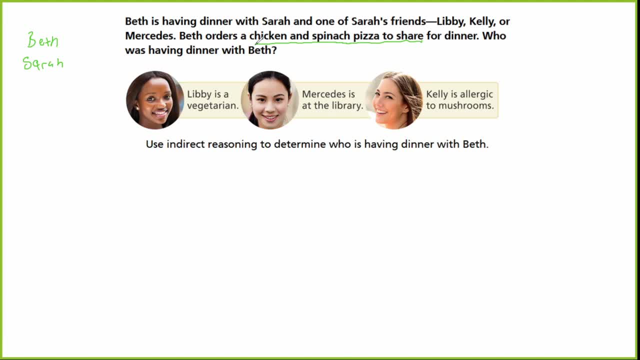 They order a chicken and spinach pizza to share, So they're all eating it. So whoever's there is going to be eating it. Libby is a vegetarian, So Libby being there leads to a contradiction of our conclusion. right, Because Libby would not be eating a chicken pizza. 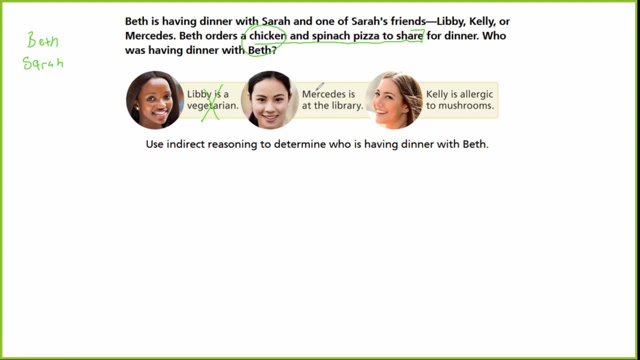 Mercedes is at the library. Um, libraries are expanding their services to survive in an ever changing world, But I'm not sure that many libraries are serving pizzas and holding dinner parties, So Mercedes being at the library probably means she's not at the pizzeria. 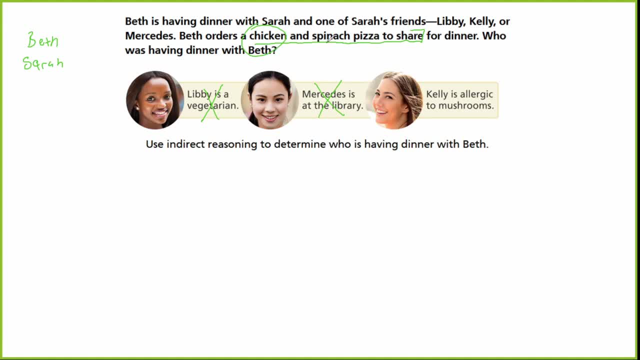 And Kelly is allergic to mushrooms. Well, there's nothing here about mushrooms, So Kelly would be safe to eat this pizza. She's not a vegetarian. Spinach is not a mushroom, So it looks like Kelly would be our best bet at the third friend. 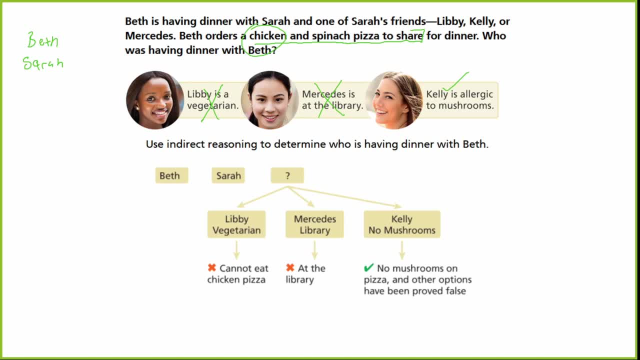 So let's see If we can do this. Well, yeah, just like we said, Libby can not eat pizza, Mercedes is at the library, No mushrooms on the pizza, and other options have proved to be false, So that is not actually a very strong standing point, right? 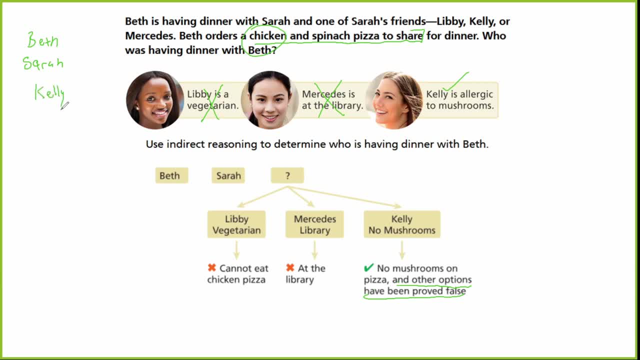 We can't just say, because we've run out of options, The last one standing is automatically right. Ideally, if you're testing stuff and you're using your education and you're bringing everything together, your last option is going to be: 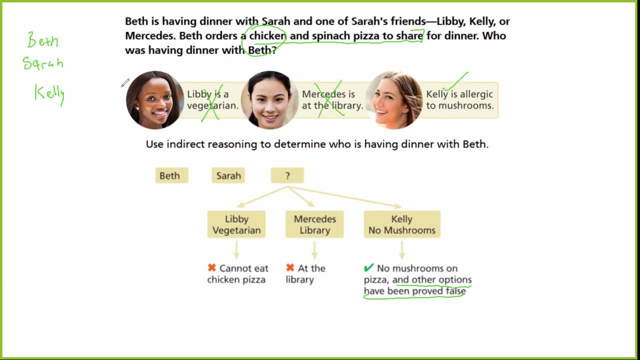 Okay, Okay, Okay, Then you're going to be the one that you've used all your previous knowledge to determine is likely the least, like you know, least likely to be the right answer. of course, here we're just ranking three friends of Sarah who will be having dinner with Beth. 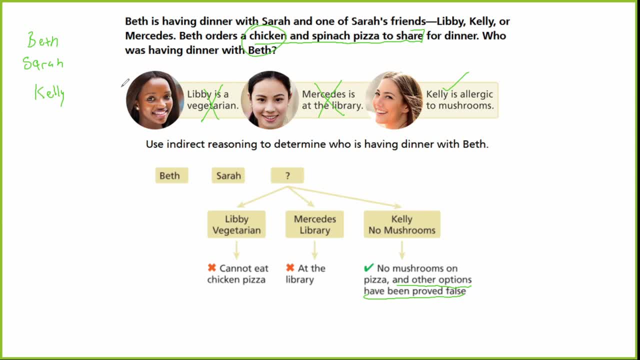 So putting Kelly last had nothing to do with the value of Kelly, but mathematically in the order that we offer them. Libby to us would be the best bet, Mercedes would be a close second and then Kelly is our last hope, right. 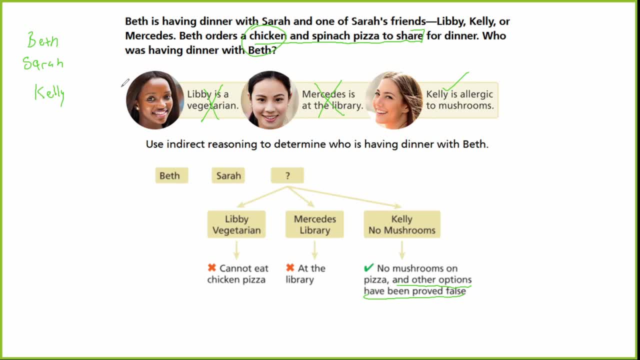 are three conclusions that we hope work. we're not completely convinced that we're. Kelly's being the third option is going to be the one, but because this is just the word problem and we just need to think through it, the order or ranking of how likely these are to be true is not impacted all. 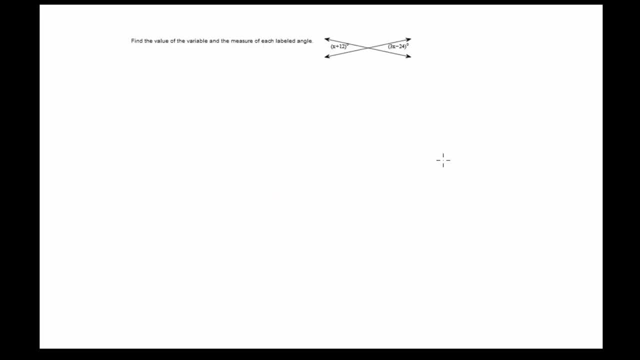 right. so let's look at our first homework problem from 1.7. it's asking us to find the value of the variable and measure of each labeled angle and knowing the vertical angles theorem, now we can say that X plus 12 is equal to 3 X minus 24, because by the vertical angle, vertical angles- here I'm 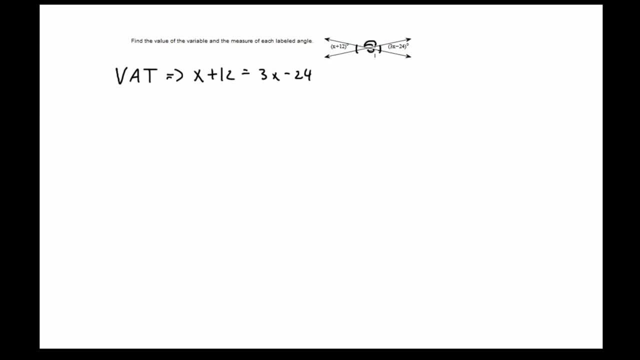 these takes, and these two are congruent as well. so if I set these equal to each other, I can now solve for x. what I'm going to do is, since I have a negative here, I'm going to move it over, especially because my coefficient in front of this x is 1, and that's not going to leave me with a. 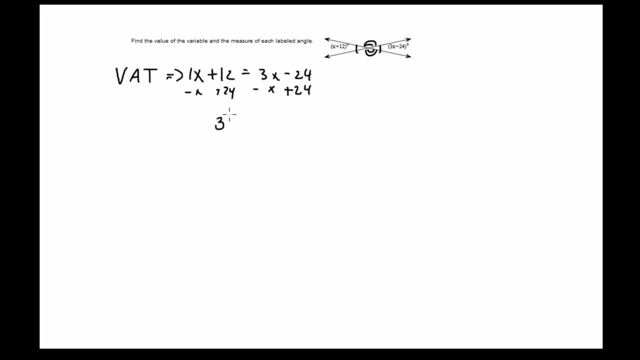 negative x. this is going to leave me: 36 is equal to 2x divided by 2, and x is equal to 18. the reason we can now do this is because we know the vertical angle theorem and we know that those angles are congruent. let me show you that one more time. vertical angles theorem says: 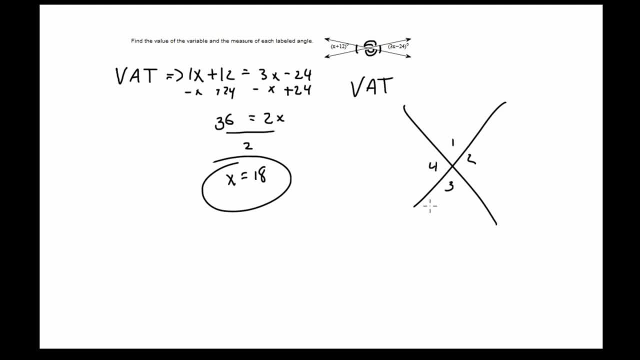 I'm just going to write them in this fashion: 1 is congruent to 3 and 2 is congruent to 4, and since that's true, we can set them equal to each other and solve for x. all right, so the answers are already on the screen for you, but let's talk about why these are the answers. 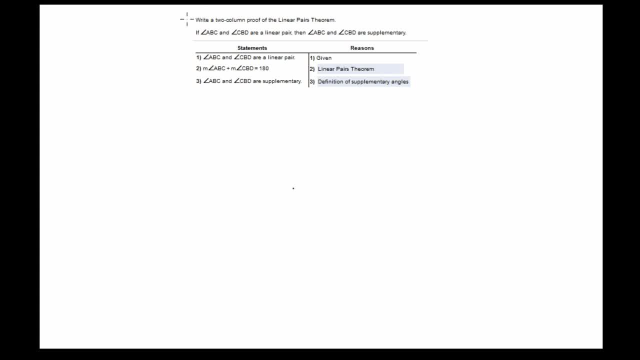 so, with the it says, write a two column proof of the linear pairs theorem. so, as we know, the linear pairs is just. if I have a line that has a ray or even another line or line segment passing through it that generates two angles, then angle 1 plus angle 2 is equal to 180 degrees. so here they've said: 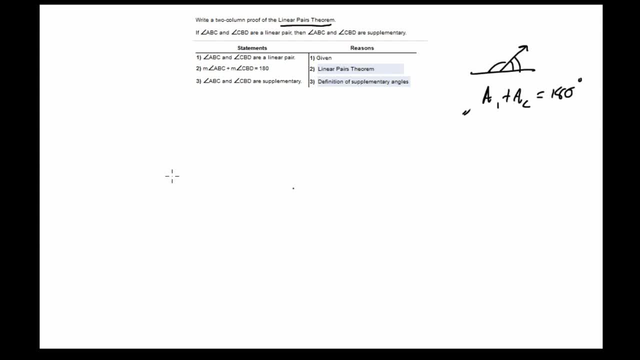 if a, b c and c b d are linear, are a linear pair. so let's label this: I have a b c and I have C B D. notice that B is the vertex on both of these. that's a really good start on making this proof happen. so now I can make this one a to be to c and then from c to be to D. 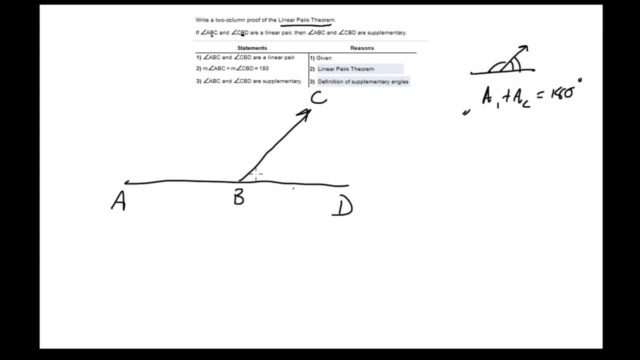 right, just set it up: our linear pairs. does this look like they're gonna be linear pairs? absolutely, I can take this one plus this one and that will give me the entire angle. So I can see now that my two purple angles added together will equal my green angle of 180 degrees. 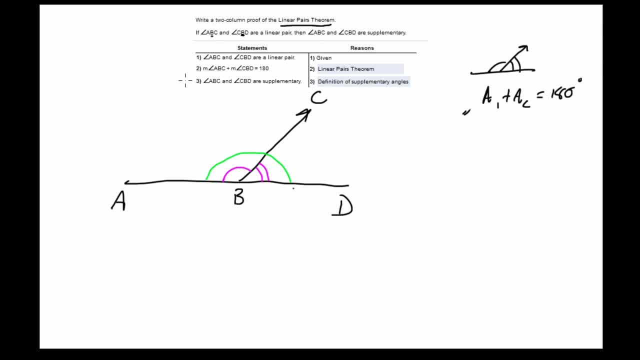 But we don't have to do all that anymore. We're just trying to write a proof. So here, visually we can see that the measure of angle ABC plus CBD is equal to 180.. We have visual proof. We've done it on this lesson already. 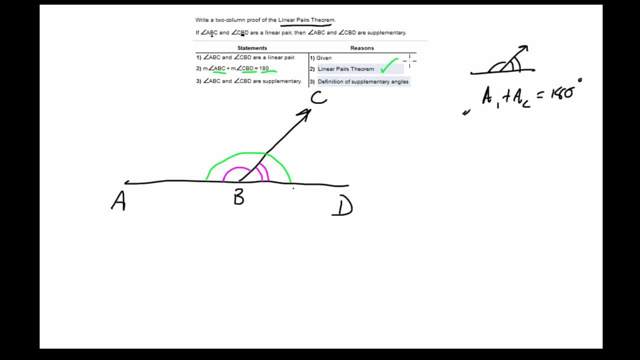 You've done it in your homework, So you can just say that, yes, by the linear pairs theorem this is true. Now, this is a slightly new thing for us. ABC and CBD are supplementary. Well, what is the measure of the angle AD? 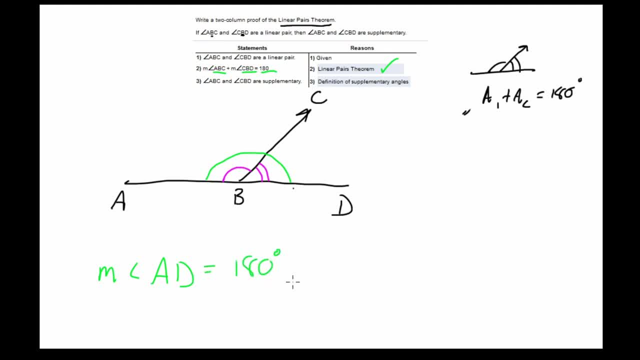 Well, in green, there we have 180 degrees And, just like we learned in our protractor postulate, I can add my first purple Angle plus my second purple angle together, since they share BC, which we can see right here, where this one ends. 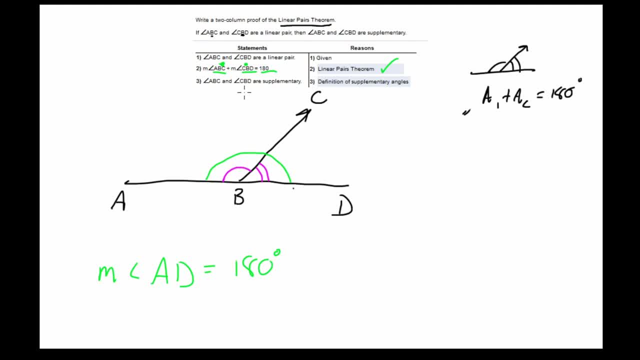 All right, BC. the next one begins CB. even though it's reverse order, we know they're the same. They also share this ray right here by my drawing. So yes, by the definition of supplementary angles, we are good to go. 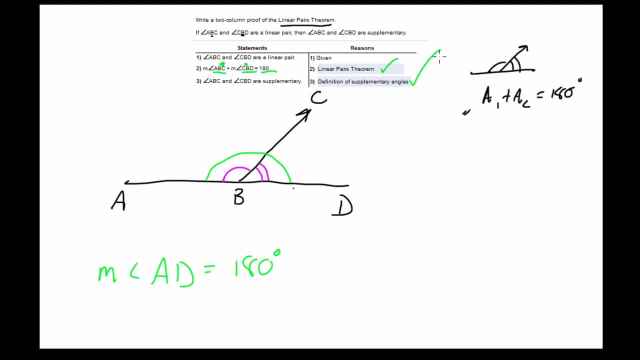 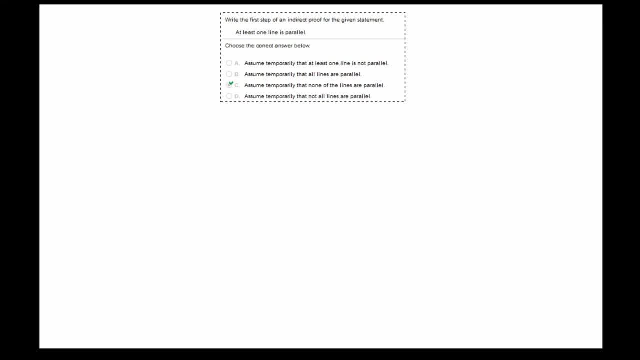 And that is your two column proof for linear pairs theorem. All right, let's look at writing the first step of an indirect proof- Remember, indirect proof is we're aiming for a contradiction, So our statement is: at least one line is parallel. 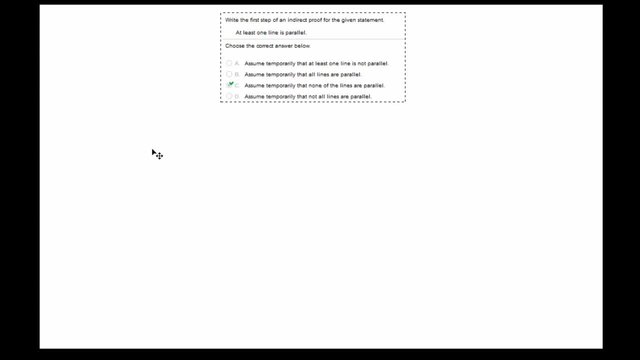 So if I have three lines, let me switch to the writing tool. So I have line one, I have line two And I have line three. So it says at least one line is parallel. How would I write a contradiction there? Well, I want to assume that none of the lines are parallel. 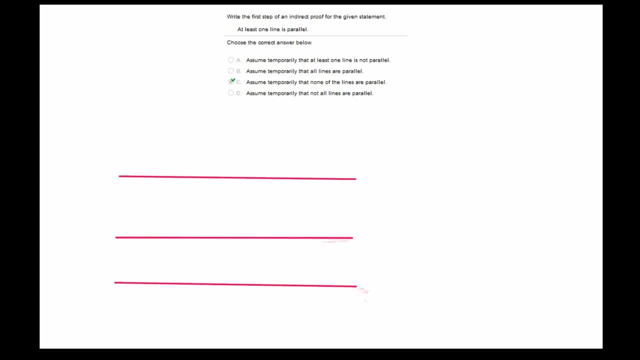 And then my task there is to show that at least one of the lines is parallel to another line or something else, And that will create that contradiction. for me, right, At least one line is parallel means if I have line one, line two and line three. 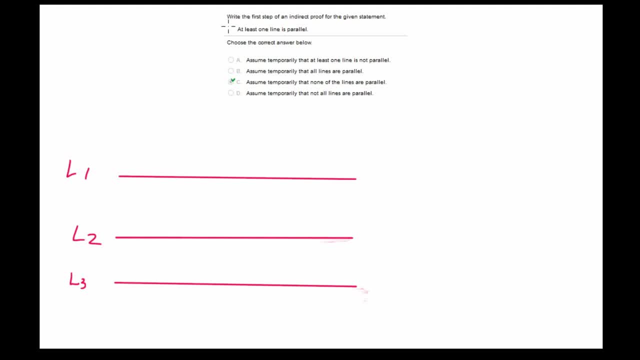 I can say: assume temporarily that none of these lines are parallel. I can say: assume temporarily that none of these lines are parallel, And then I'm going to show that they are in fact parallel, And to do that I can use a theorem that we'll learn in the future, but I'll show you really quick. 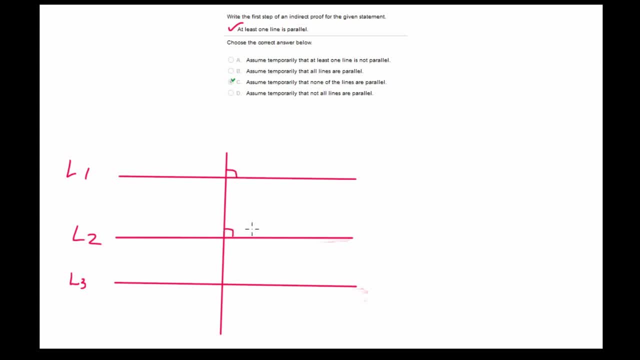 It just says if two lines are perpendicular to the same line, then they're parallel to each other. So since line one is perpendicular to line four and line two is perpendicular to line four, then line one is parallel to line two. And if you think about that, wherever you're sitting right now, 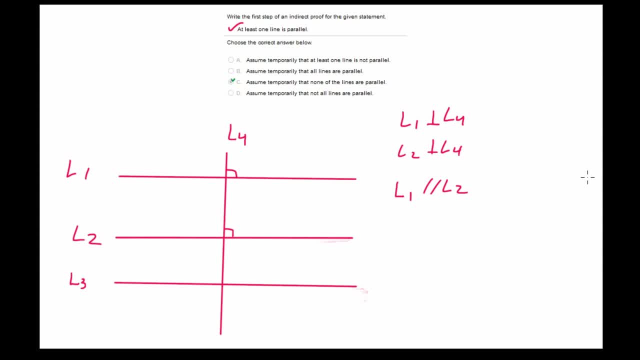 if you have a door or a window nearby, this will work. This also works. you're obviously watching this on a computer If you look in the top right corner of your screen, right up here. if I were to call this a line, 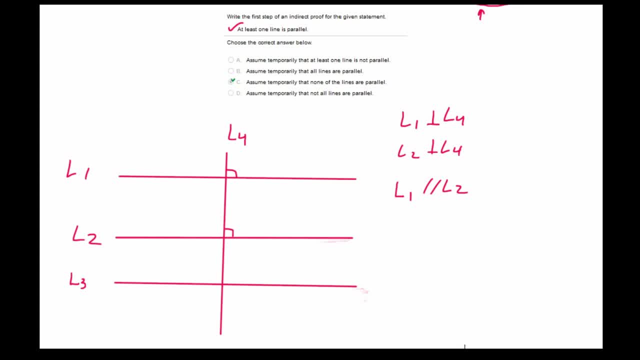 it's parallel with the very bottom of my screen, But if I go to the top corner it's perpendicular to this vertical line. And since the top line, going horizontally, is perpendicular to my vertical line and my bottom of my screen horizontal line is perpendicular to the right hand side as well. 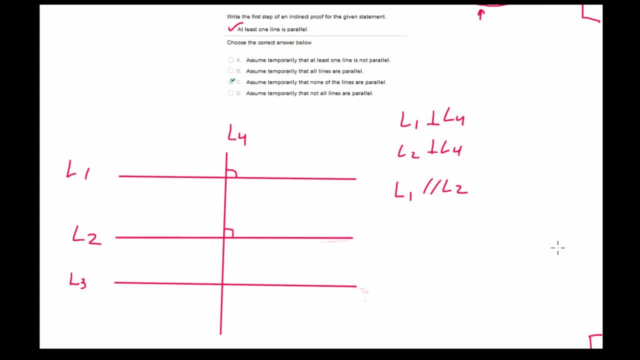 then my top and bottom are parallel to each other. That's all that theorem tells us. That's actually called theorem 2.9.. And that one is definitely on your writing assignment. It's also on the proof video that I show you on how you can take one picture and pretty much find. 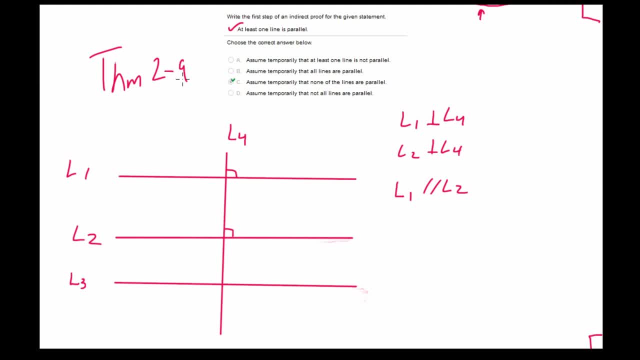 any of the proofs that I'm asking you to find in just about any picture, But we'll definitely go over that more in class when we get there. But here we can now show that these lines are parallel and we've set up the contradiction, so at least one of the lines is parallel. 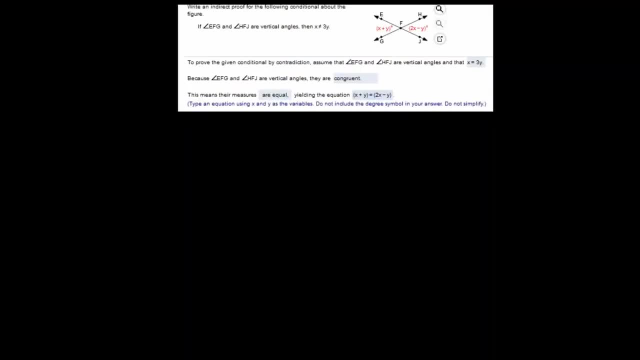 All right, here's another one for indirect proof. I want to keep practicing these because these are very important. These are your contradictions, And what it says is write an indirect proof for the following conditional about the figure. So here's what we're actually looking at when we're doing this problem. 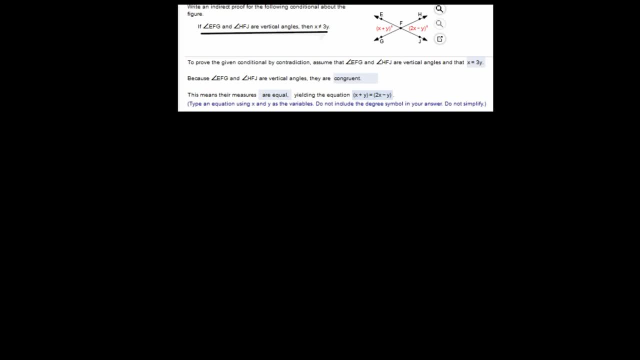 And it says: if EFG- so that is from E to F to G and H to F to J- are vertical angles, which they are right. This hypothesis is true By the vertical angle theorem. they're going to be congruent. 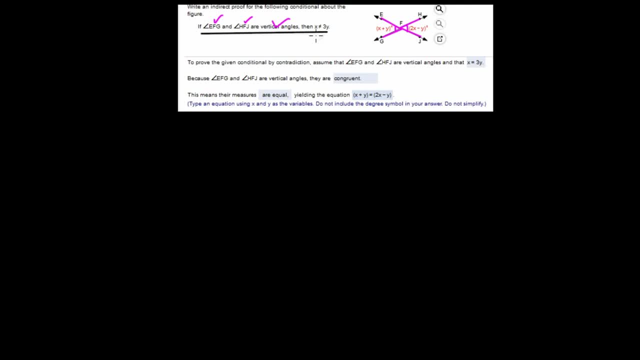 So we can say that's true because of the way that this diagram was drawn, Then X does not equal 3Y. So remember, we want not Q for our contradiction to be positive, We want to make that contradiction possible And then, once we can show that the contradiction happens, we can then say that the overall value is: 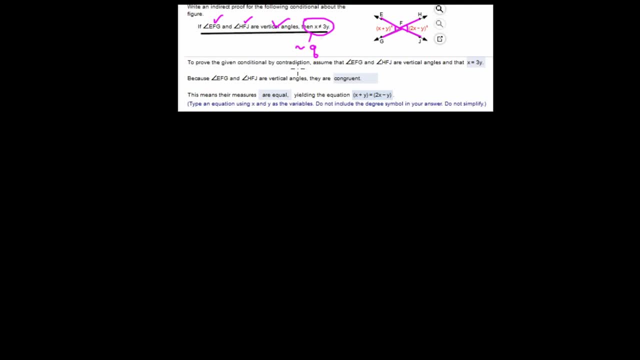 true. So to prove this, given conditional by contradiction, assume EFG and HFJ are vertical angles and that- and look here- X equals 3Y. So that is the negation of X does not equal 3Y, right? What's the opposite of does not equal, It is equal. 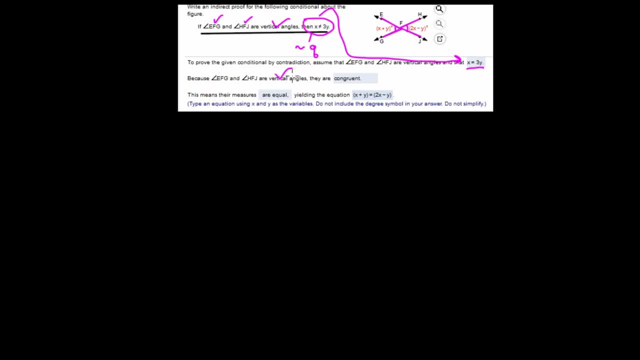 Because EFG and HFJ are vertical angles. again from our hypothesis, they are congruent and we're going to say, by the vertical angles theorem this means their measures are equal, again by the vertical angle serum. yielding the equation x plus y equals 2x minus y, and what we need to do now is a little bit of algebra. 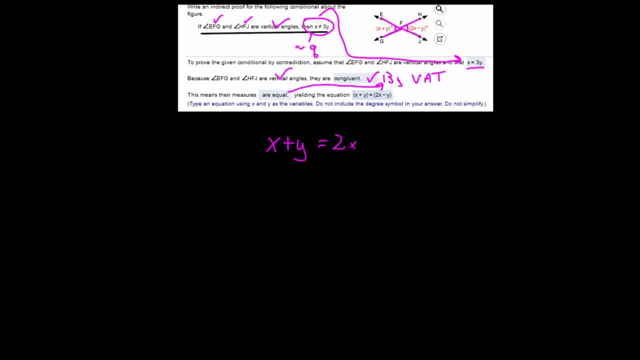 but notice now that we're in geometry, they're not actually asking us to do that. this is what they call in higher level math classes. this is a trivial piece or this is a exercise left for the reader. never again, until you get into much higher level math classes, will your teacher say, let this. 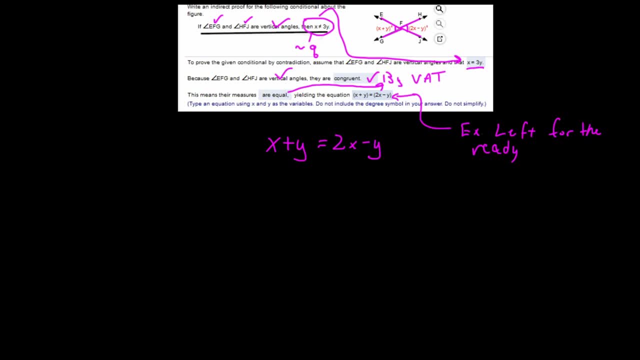 be an exercise for the reader if you get to this point. this is algebra one, pre-algebra stuff. it's just manipulating the equation. i am okay with on your writing assignment saying an exercise. this is an exercise left for the reader. i wrote ready. let's uh, just pack that one out there. 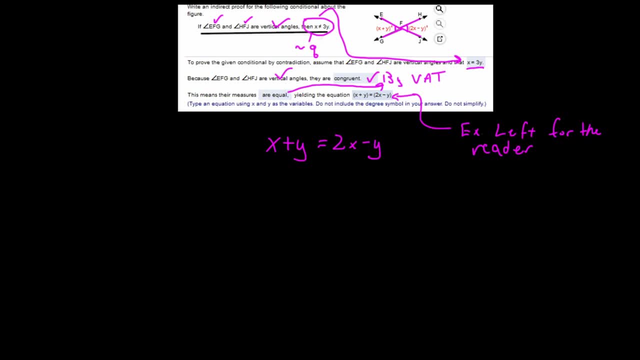 all right, but i'm gonna go ahead and show you that, go ahead and show you what this looks like when we balance it algebraically. so i'm just gonna show you that this uh looks like algebraically. i like this. i'm going to show you what this looks like algebraically. 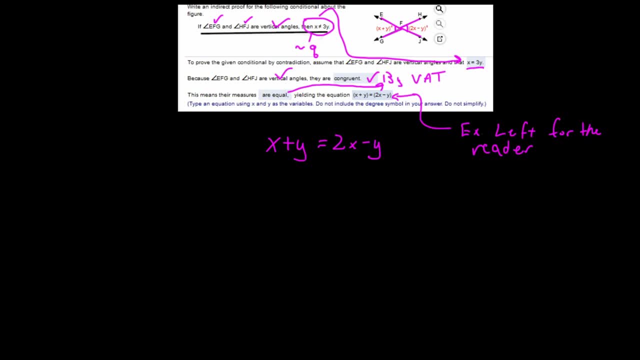 so i'm gonna get my x's by themselves, but i want everything to be positive if i can. and that means if i move this over, i'll be left with that just X, and if I add this over, I'm just left with plus. oh sorry, plus Y gives me. 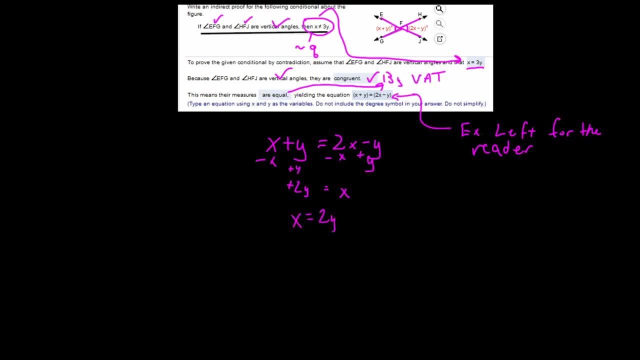 positive: 2y. X is equal to 2y. so we have a contradiction here, right, we said so. here's our contradiction here. our negation said: X equals 3y, which does not equal, and we have shown so. here's that word. we again by a contradiction that, and we just rewrite: 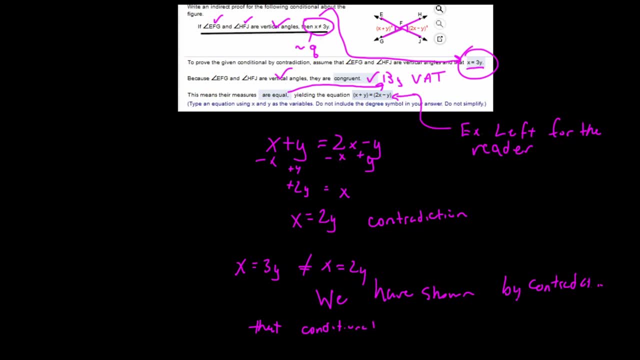 the conditional is true. now do we have a full-fledged theorem here? no, we have not shown this for all cases. all we've proven right now, all we have actually done, is show that X does not equal 3y. but that is an indirect proof for this problem as it's written for us. so at 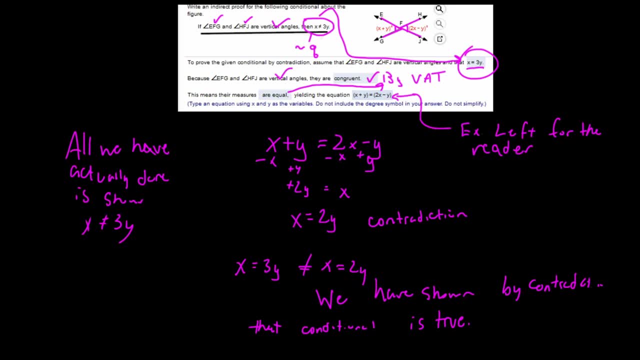 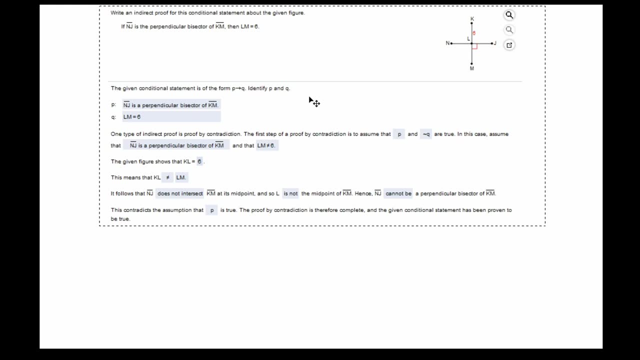 least we have that done and we can move on to our next problem, and we're gonna look at one more. write an indirect proof for this conditional statement about the given figure. so our hypothesis is: if NJ is the perpendicular bisector of KM, so this is P. 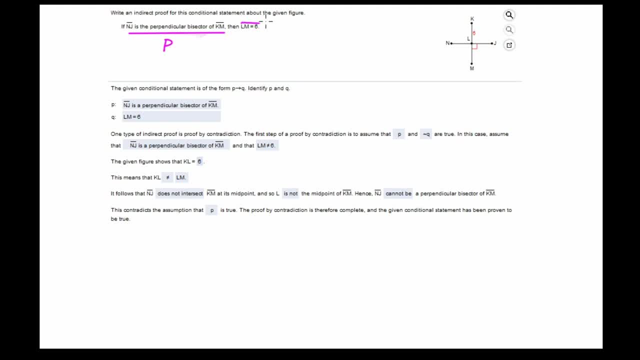 and Q is LM equals 6. so right here it's asking for the given and that's why I'm not negating anything yet. identify P and Q as it's written. so our P we just bring down here, our Q we just bring down here. double check that. I filled that out. 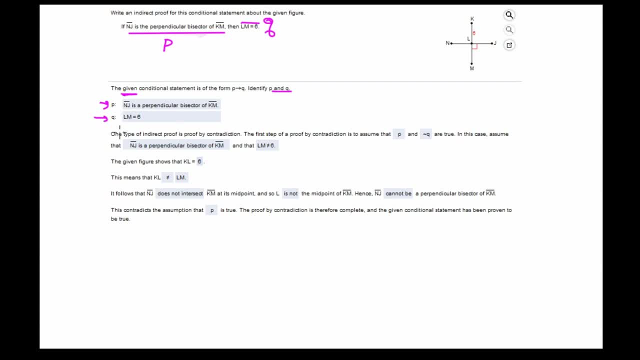 correctly. we're good to go. one type of indirect proof is proof by contradiction. I know I keep saying we're gonna use proof by contradiction as indirect proof. that is our main one. we also have contra positive and a few others, but you're not going to need them for this course. I'm actually editing out most of those. 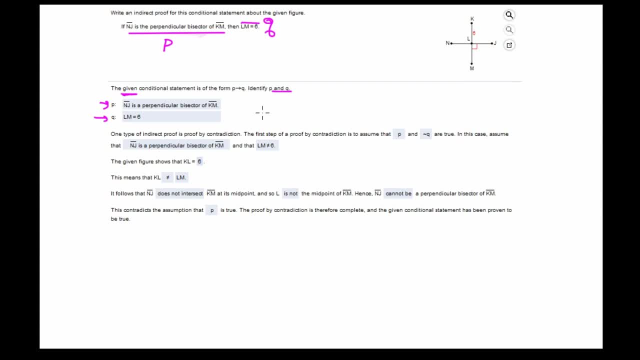 questions because we are missing a week in this school year, so you don't have to worry about that. so the first step of a proof by a contradiction is to assume that P is true, or assume P and not Q are true. so that goes back to our 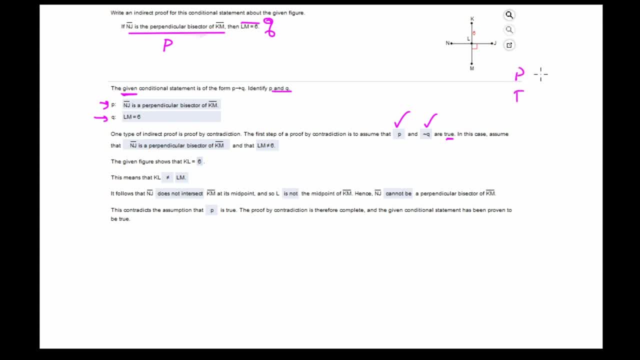 truth, truth table and we want P is true and not Q is true, but we need to show it's false so that we can get that the overall truth value of this is false and therefore our original conclusion is potentially true. so if, in this case, assume that NJ is the perpendicular bisector of KM, we did not change our 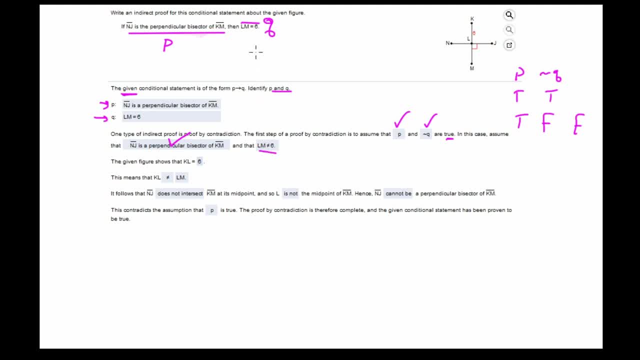 hypothesis, but we did negate our conclusion. LM equals six negated. his LM does not equal six. the given figure- so this is part of our hypothesis here, because it was given- is that KL equals six. this means that KL does not equal LM, so all to him. so we 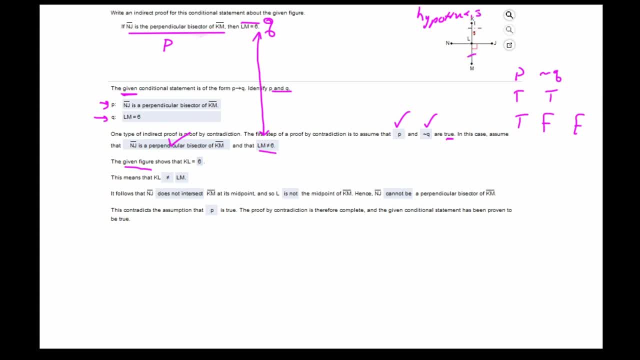 can. what it's saying here is: I cannot put a tick mark on either one of these. if that it follows that NJ does not intersect KM at its midpoint, so this is the caveat there that we can say it does not happen. so L is not the midpoint of. 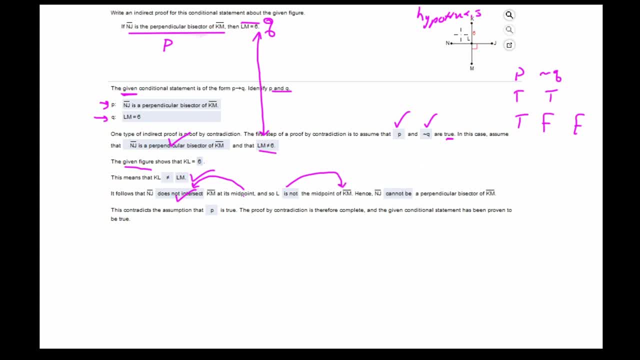 KM and NJ cannot be the perpendicular bisector of KM. now, we don't know the word bisector yet. this is why I have this as a homework help problem. the bisector means it cuts it in half by means to and sector. by means to and sector. 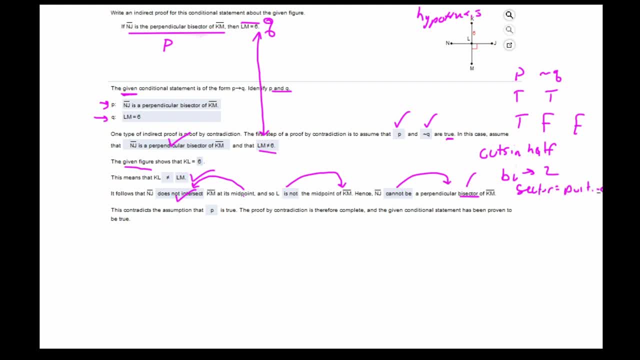 by means to and sector. we'll just call portions for now. so bisector means two equal halves and basically this whole proof is saying that if we cannot say that these are true, then this cannot be cutting it in the middle. it is the perpendicular interceptor but it's not the bisector. this contradiction contradicts the 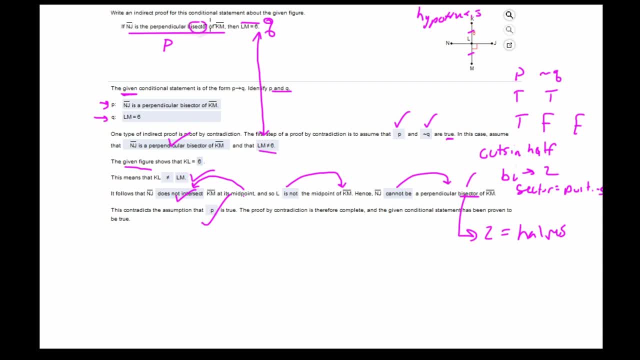 assumption that P is true, NJ is the perpendicular bisector. the proof by the contradiction is therefore complete and the given conditional statement has proven to be true. so, basically, this whole problem boils down to this: points point P, point NJ, points. this whole thing sounds wrong, alright, So let's look at what exactly? what NJ? That's this guy right here.